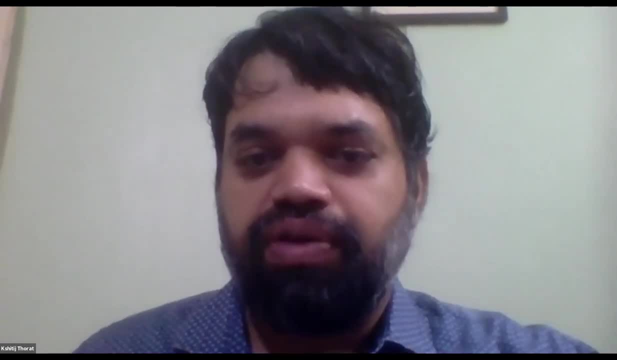 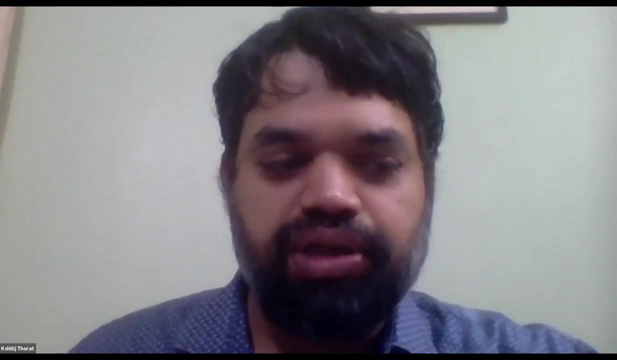 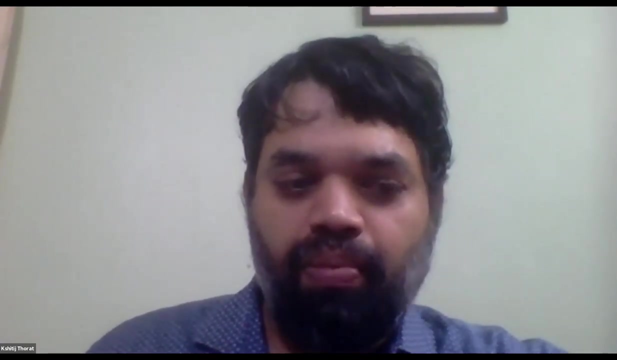 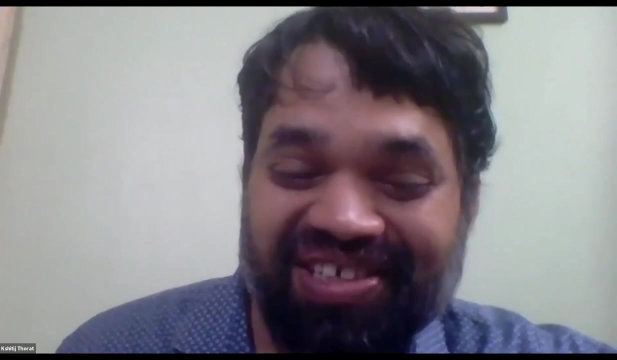 And at the end of the talk there was an iPython notebook which was shared with all of you, and Victor is going to show us how to do the exercises which were given in that notebook. Over to you, Victor. Thank you, It's actually over to Stephen. Stephen will show you My apologies. It's over to Stephen actually. 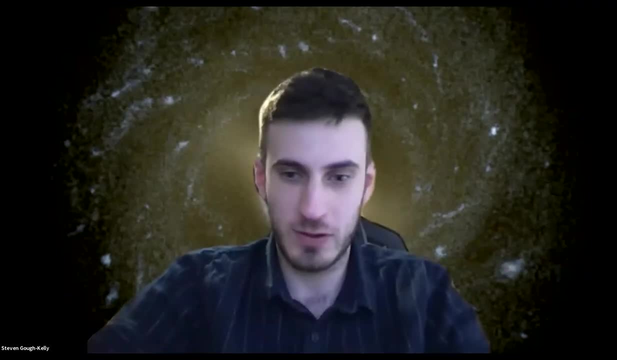 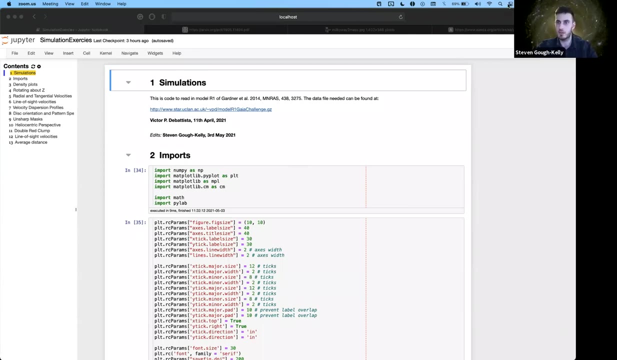 No problem. No problem at all, Cool. So I'm going to start Sharing my screen. Hopefully you guys can see my notebook. Do we want to quickly introduce Stephen? Introduce myself: Well, yes, Stephen is my PhD student and he spends a significant part of his time analyzing simulations. 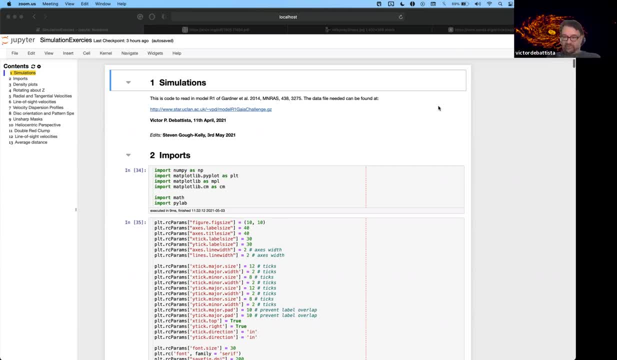 So we thought he would be a perfect person for showing you the answers to some of these questions, So I'll hand over to Stephen. Thank you, Victor. So yeah, like I said, this is my bread and butter, day in, day out. 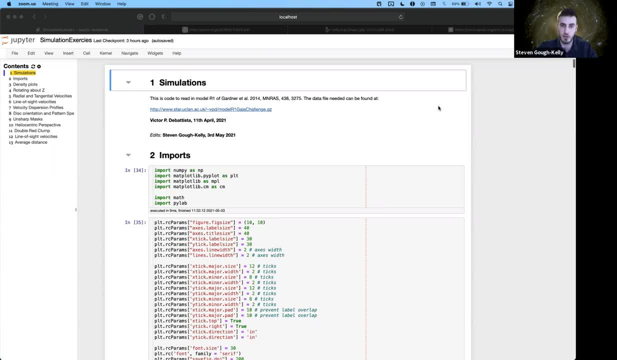 I kind of am handling simulation files and doing some level of comparisons to the Milky Way, which is what this NBody model was kind of run for. So I'm going to show you how I've approached the problems from kind of how I've from my experience. 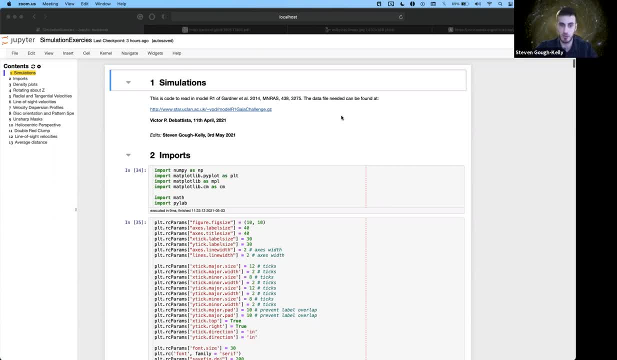 And try to kind of step through some of these examples, Showing you kind of under the hood, Stepping through some of the processes in a bit more detail than just using a library to brush over some of this stuff. I have used some extra ones than the original ones that were imported by Victor. 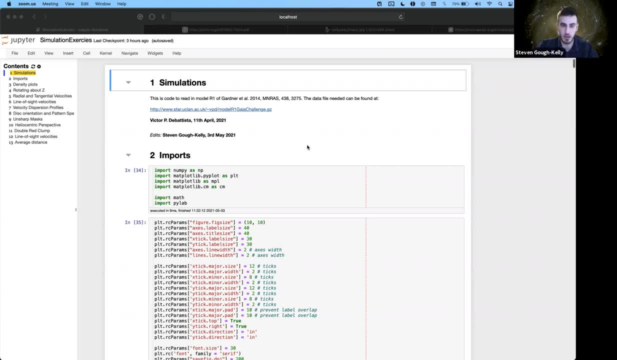 But they're fairly common And they just help with some lower level kind of iteration stuff. that is a little bit boring. So I'm going to step through each of kind of the problems And show you kind of my results And how I approached it. 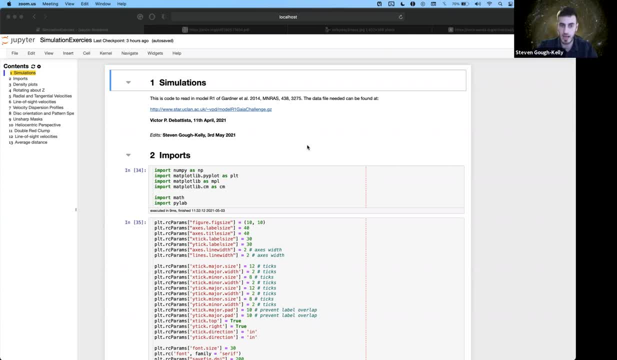 And how you can approach the same things, As if you've kind of not attended these examples yourselves, But then hopefully some of you have, And then once I've finished, I'll invite you guys to kind of share any difficulties or any things you've noticed as I've talked through these exercises. 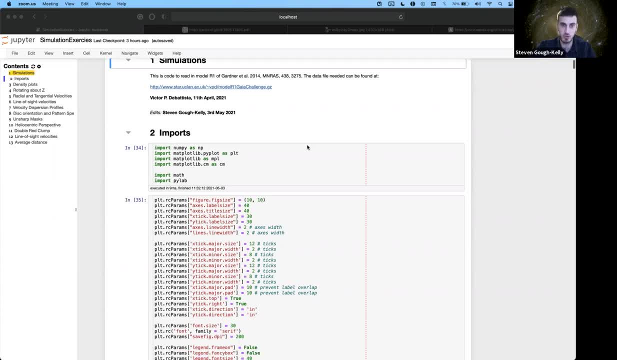 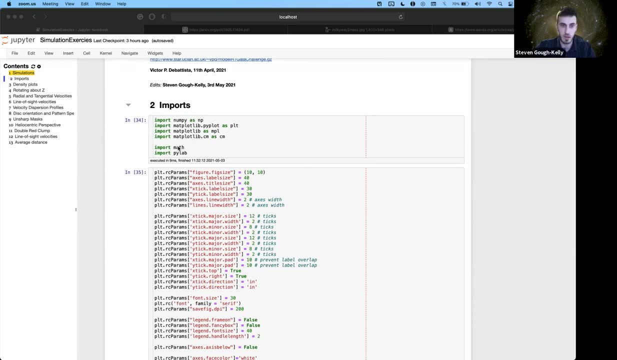 That you might want to bring up and ask questions about. So I'm just going to jump straight in. So we have the basic imports of NumPy and Matplot. Just allow us to Produce some figures, Some math functions And PyLab. 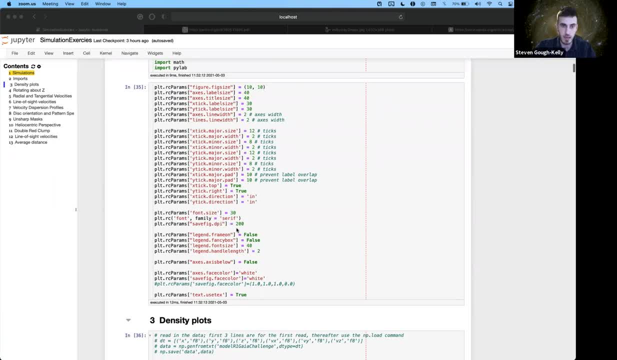 Just to help. some extra bits on Matplotlib. These are just some plotting parameters that make the plus look a little prettier, Just the labels and things like that. It was just to help me out so that when I show you a plot, the axis labels are picking up so you can see them. 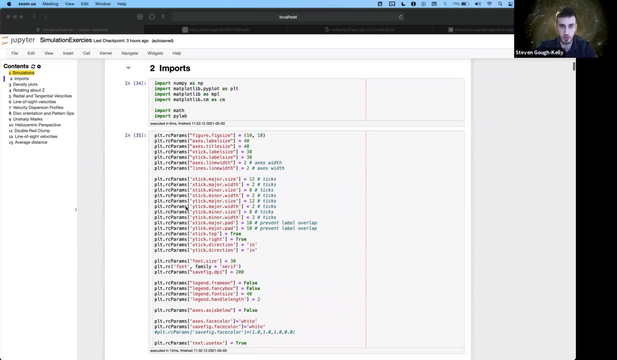 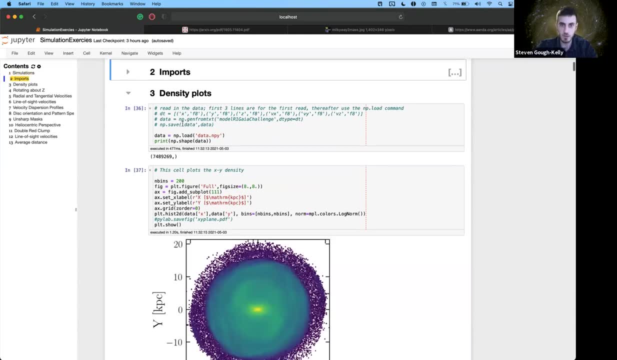 And I'm not squinting and zooming in and things like that. But we don't need to really worry too much. There's nothing fancy going on here, Just some making the plus look pretty. So Victor introduced the notebook at the end of the session. 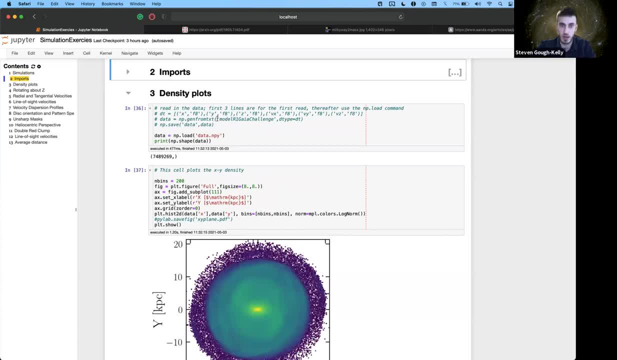 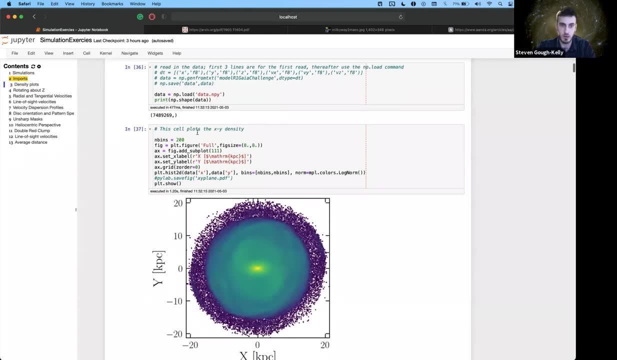 So we had an original kind of text file to begin with, Imported it, Saved it as a NumPy array And we loaded it And we're going to do some basic density plots. So we're plotting a 2D histogram of the X and Y data. 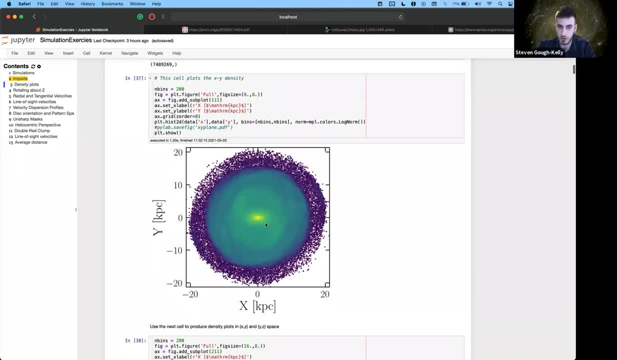 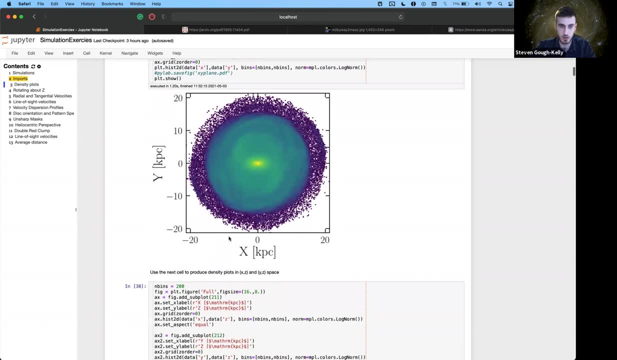 Where the colors: the more yellow it is, the higher the density. So the galaxy has the highest density in the center And we get this disk, Some level of starting to see spiral patterns. We look in the XZ and YZ planes. in XZ At the moment, if we look in the XY plane, the bar which is at the center of the galaxy is lying along the X axis. So we look in the XZ plane, We see the X shape, or the boxed peanut shape that some barred systems grow. 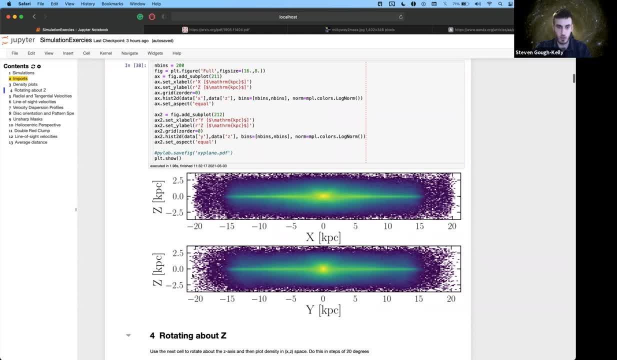 So you can see it quite nicely defined there In the YZ plane. we're looking at the bar end on And because the X shape is the vertical extension of the bar, we see at its end that we don't see an X shape. 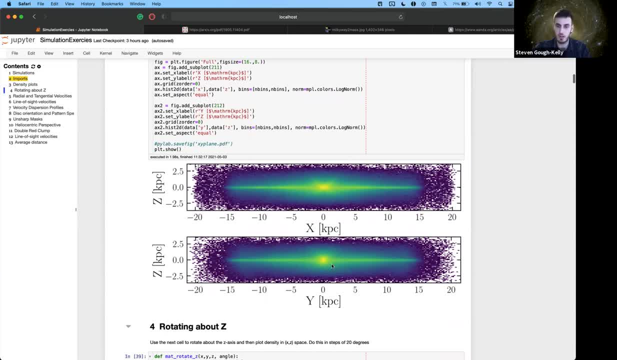 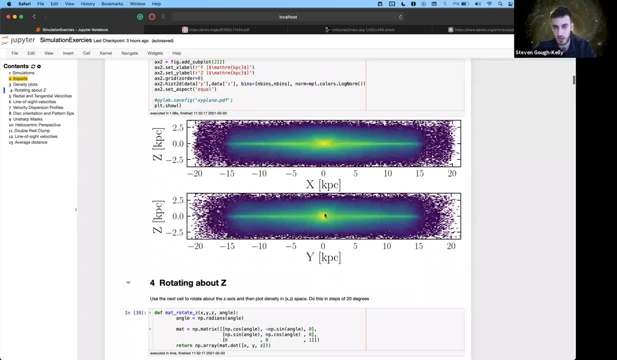 We see just more of a spheroidal distribution, Which is what we'd kind of expect. And this is a problem sometimes: that if we're looking at galaxies in the universe, if we look at an edge on galaxy and we see just a central kind of spheroidal region, it's very difficult to determine whether this galaxy is. 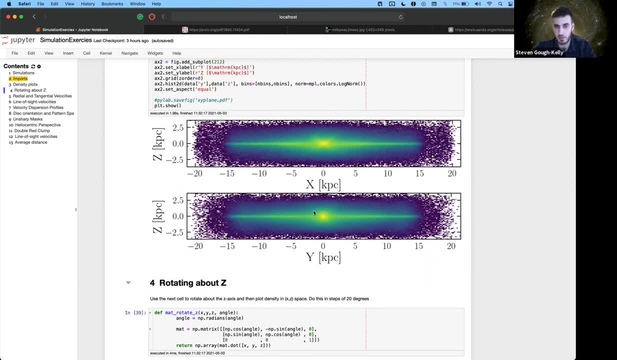 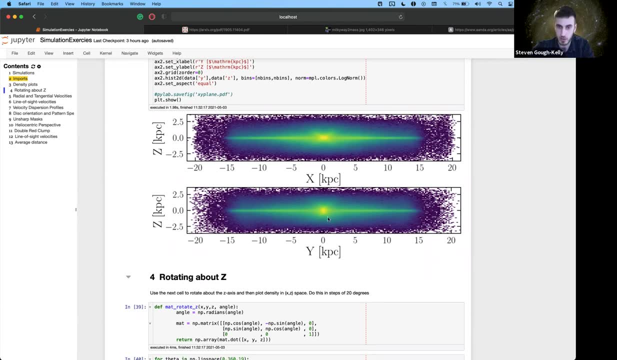 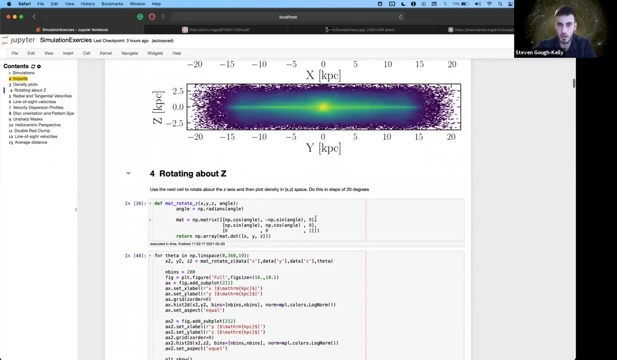 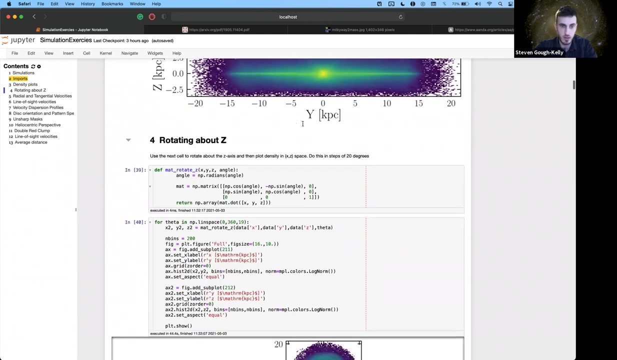 barred or we're just seeing, we're just looking at the end of the bar, Or there may be no bar in the system at all. You can't always see that just from the density distribution of light from the galaxy. So we're going to look at this kind of projection of the X shape as we start to rotate the galaxy about the Z axis. 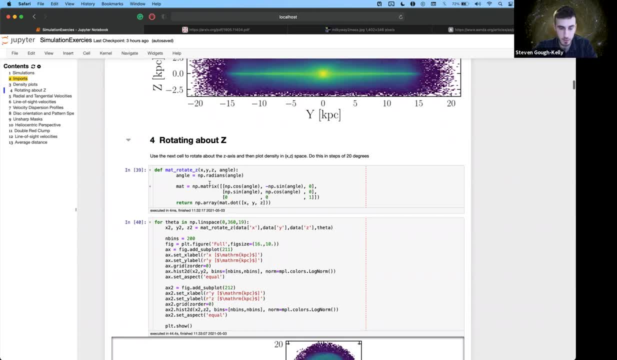 So just very simply defined a rotation matrix Using numpy. This is about the Z axis, So you give it the XYZ values And then an angle. We're using radians, So I've written it so that you can just put a degrees angle in and then you convert it to radians. 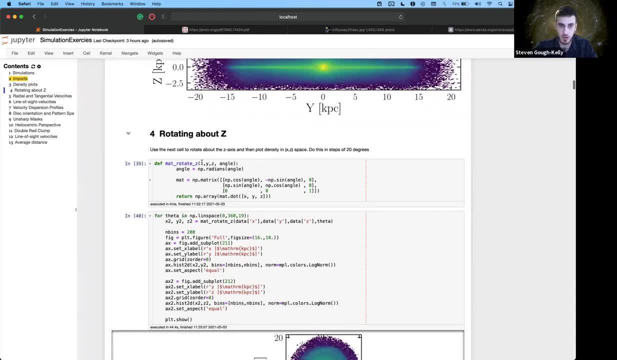 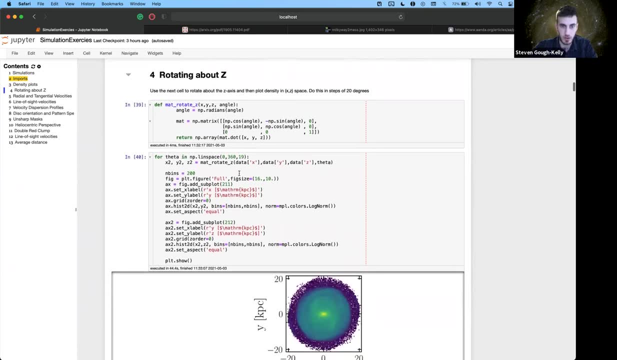 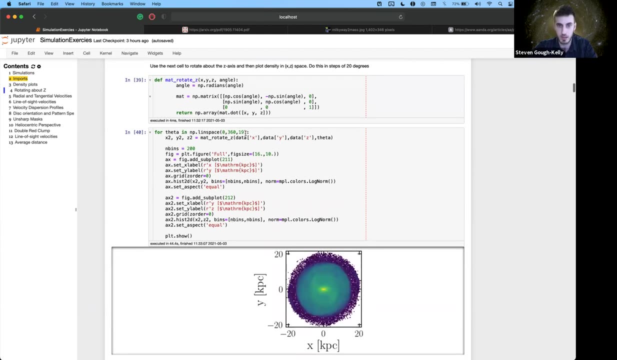 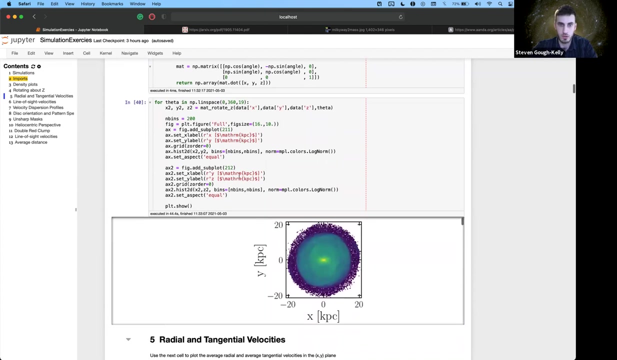 Very simply, just do the dot products with this matrix to return a new XYZ rotated by an angle. So then, very simple, for loop, I'm doing Angles within zero to 360.. 19 different bins Gives me rotations of 20 degrees. 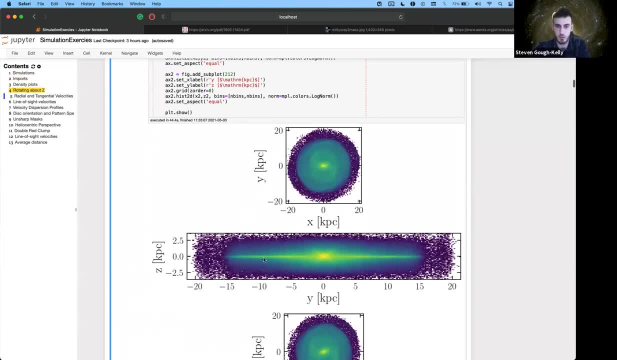 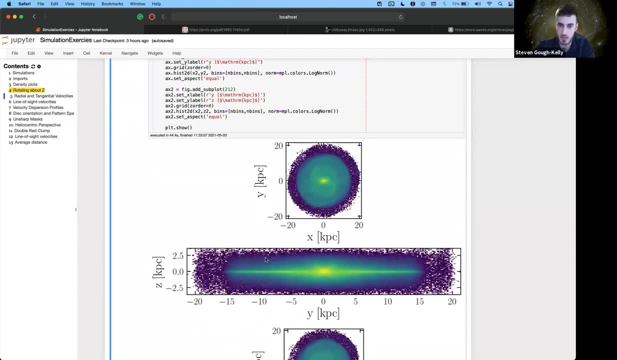 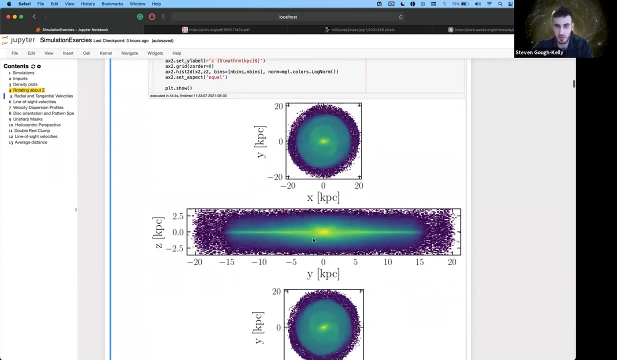 I plotted the XY And YZ. that might be incorrect. apologies, that's XZ. That's my labels actually, so I've made them big so you can see them and put them on label. This is the XZ axis. apologies, You can see, the bar is on the X axis. 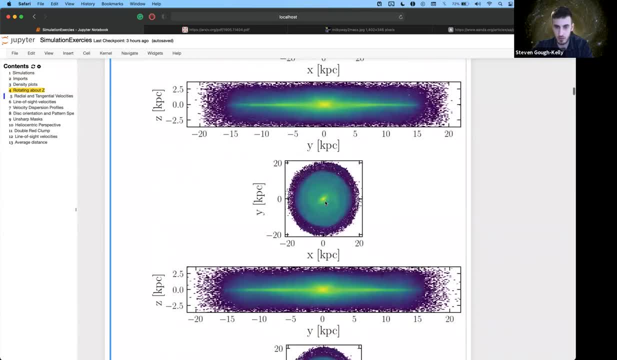 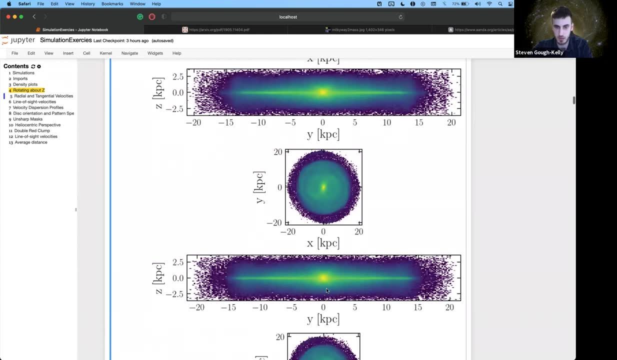 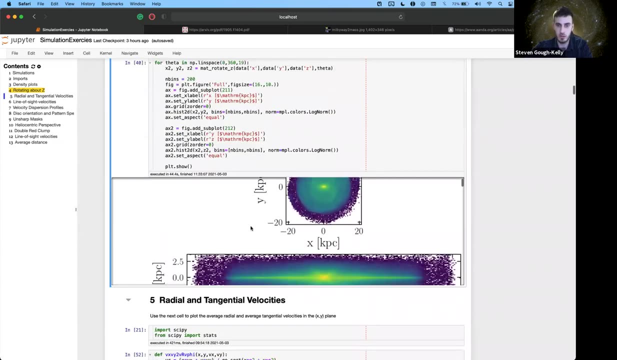 We see nice egg shape as we start to rotate through, And we will take through to where the bar is in line with the Y axis. instead, you see the X shape was disappeared And it rotates all the way through a 360.. Very simple for it, just so you can. 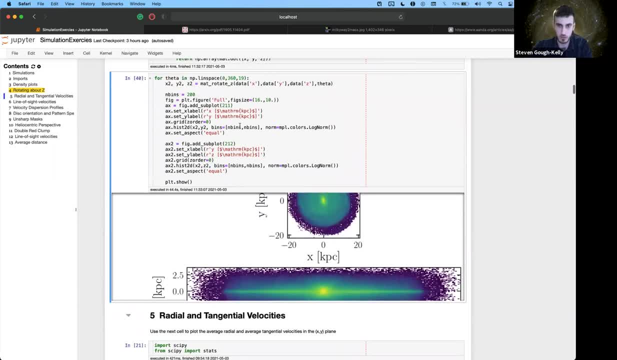 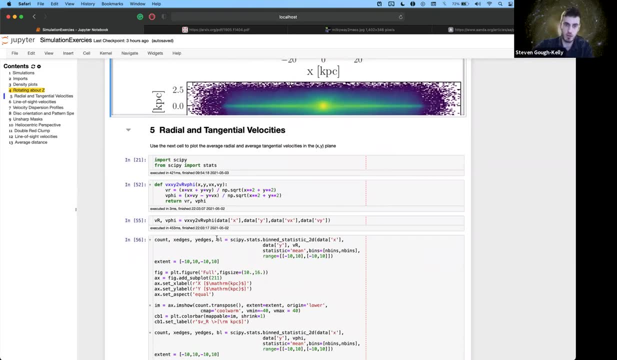 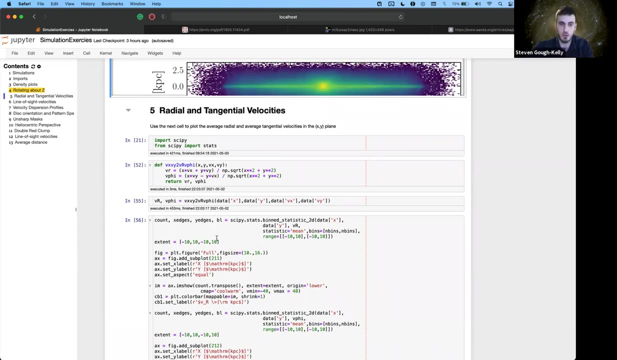 Look through all the different bar orientations. Now come Become important a little later on. Next we're going to look Just the velocities, looking at Maps about privilege velocity. so we're looking In the XY plane, so looking from the top down onto the XY plane. 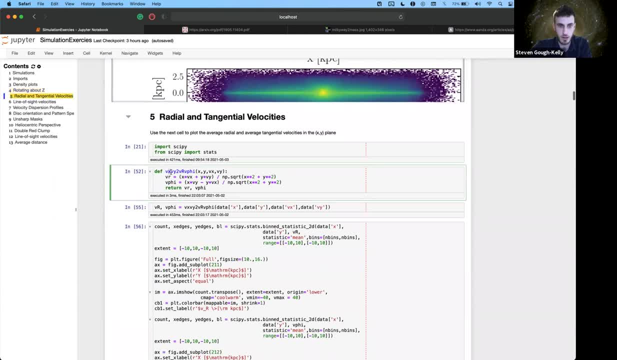 And I've done a very quick definition of The XP, why, Converted to radio velocity With respect to the galactic center And the tangential divorce velocity, be five, which is about the galactic center. So I just very quickly define those. 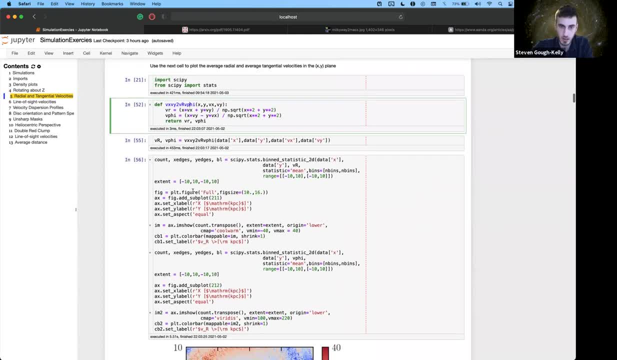 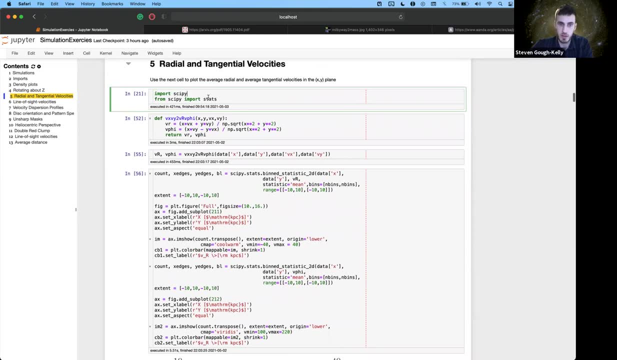 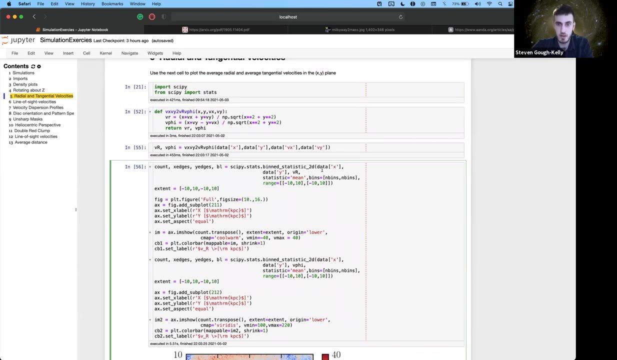 We got the RP fly And then I've changed the Binning routine that I've used. I've Imported a package side by And from side by you've got the stats Functions And within stats it's got this nice function called been statistic 2d. 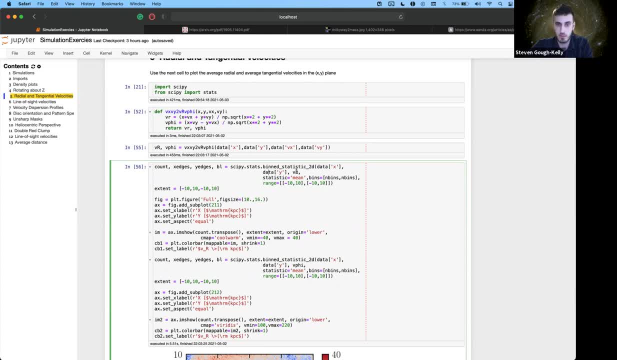 You give it the two dimensions, the X and Y data, and then you give it the third dimension that you want to Histogram. You want to Bin The data And give the And give the color or the Z Access. 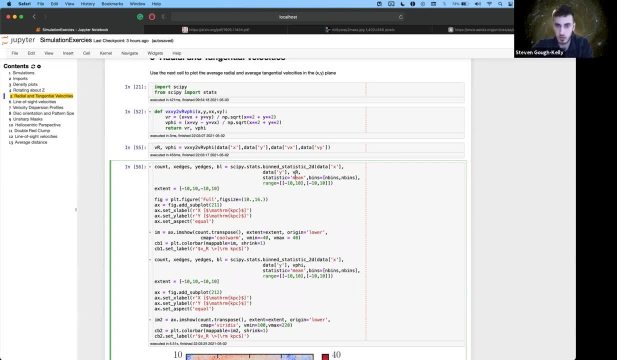 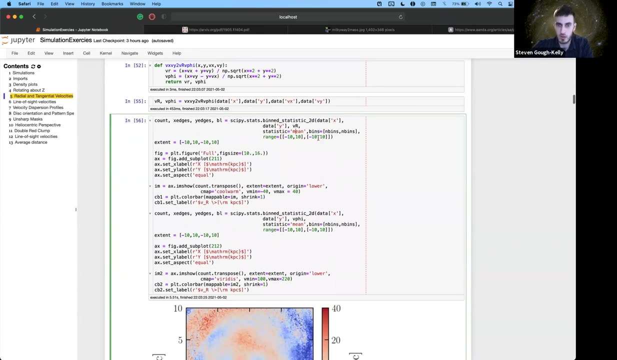 Which property you want to do that. Which statistic am I using? you can do things like count, so you can make it adult, The third dimension, or you can make it do an average or a standard deviation. I tell it the ranges. and So what? what area of the galaxy I want to call the X and Y data in the number of bins. 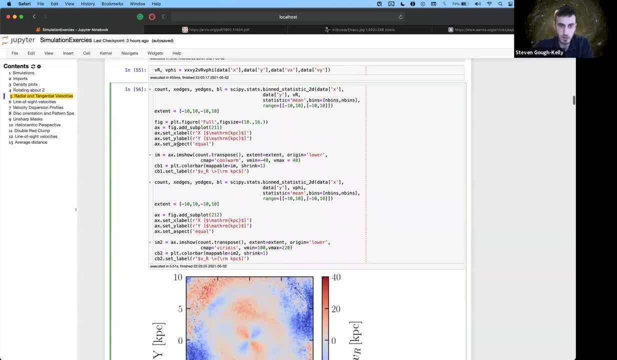 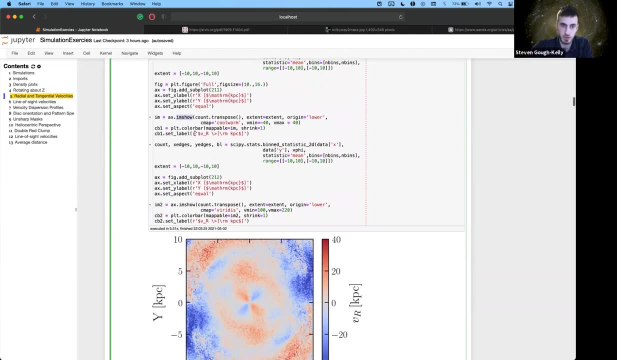 So I'm using the same number of things before, Very simply just setting up a new plot and using In show Which just takes a 2d, 2d array of values And And produces the image of it, Adding color bars or nothing. 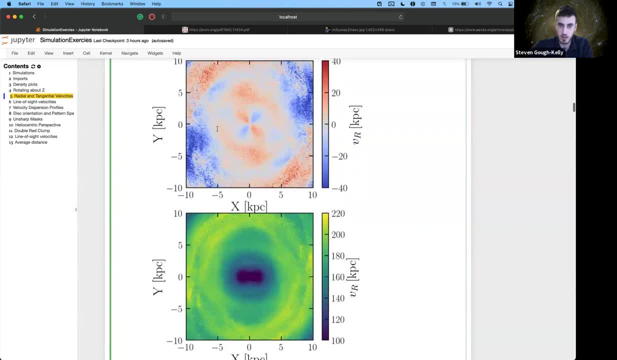 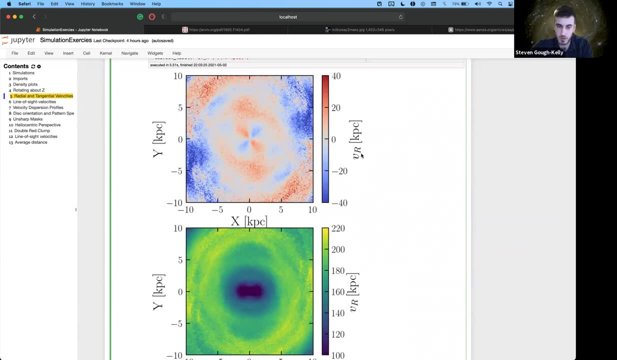 Too extravagant, Which gives me these two plots. So in an X and Y Range You've got the average VR. It should have average marks and those. apologies, but this is the average VR. So In a square, In a square bin. 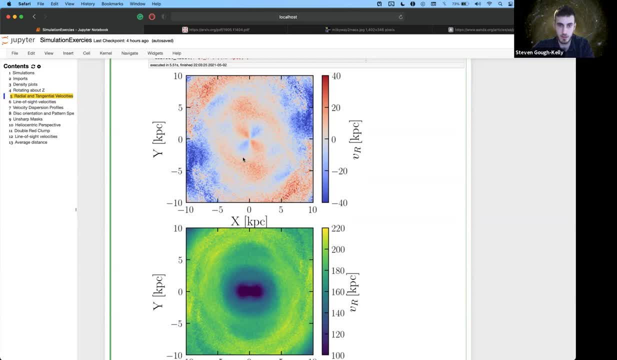 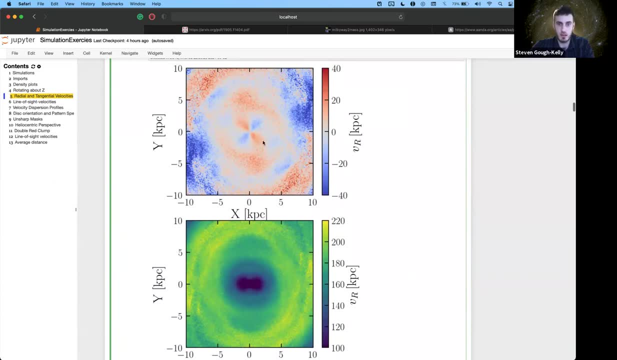 So many, So many. What's the average VR value? And this is what we get out And this is kind of what we would expect for a bar galaxy. You see this nice quadrupole butterfly kind of pattern in the center Which is kind of indicative of the bar. 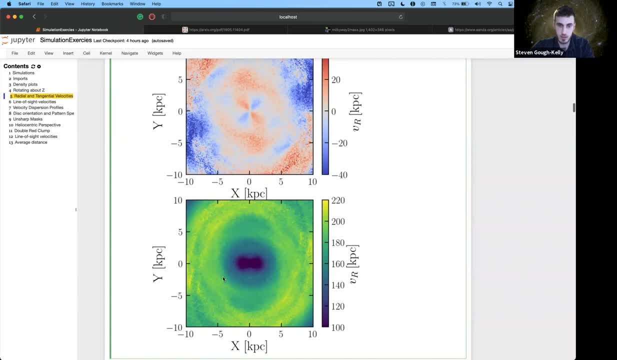 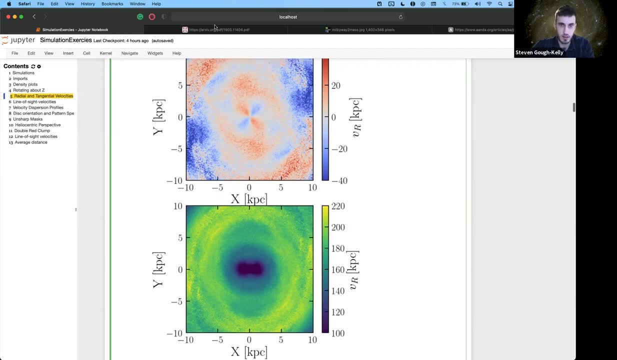 You got quite high tangential. He's quite near the center. Sorry, Low tangential, This is near the center And high values out in the disc And And We'll see Next one I have, I Open- of a paper. 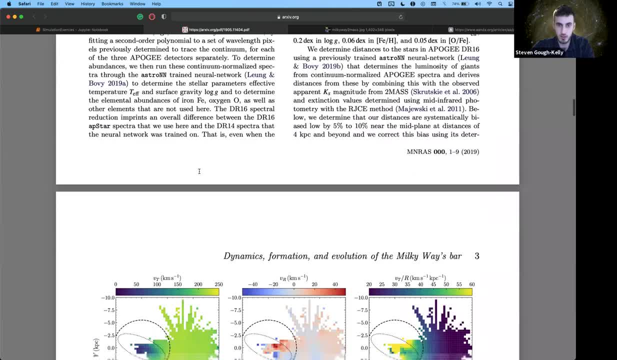 This is by Bovia, I think it's 2019.. It is Yeah, Like in the past, and then it's called: This is from. This is Gaia VVV data And you can see the tangential velocities and the radio velocities here. 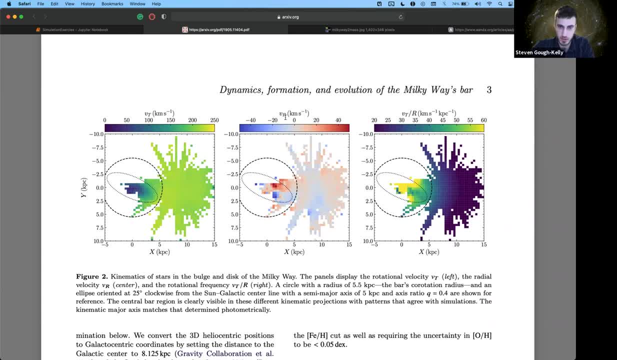 You can start seeing The same. So far, some low tendence Pluses near the center And the Other out. This beginnings of what is to be kind of a quadrupole pattern. near the center Is the same, So 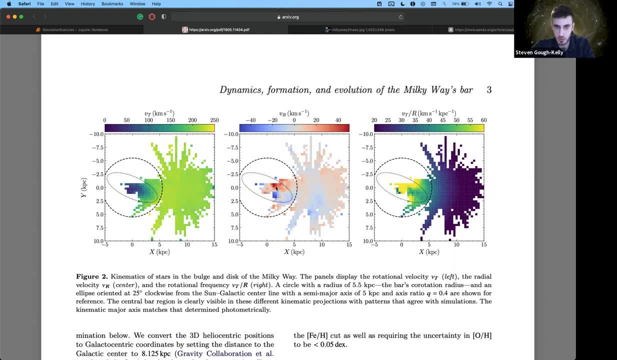 It's a funny, It's a. It's a. It's near the center, but observationally within the Milky Way it's hard to get really deep beyond the galactic center. The sun is over here at eight kiloparsecs roughly. 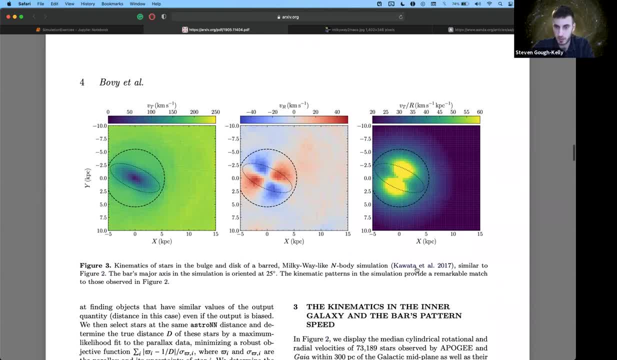 In this paper, they used another M-body model from the Palau Hotel 2017 and again this kind of reproduces these patterns that we're seeing in the data. So this is a good sanity check to know that they're kind of doing the right thing And also not to plug my own work, but this is 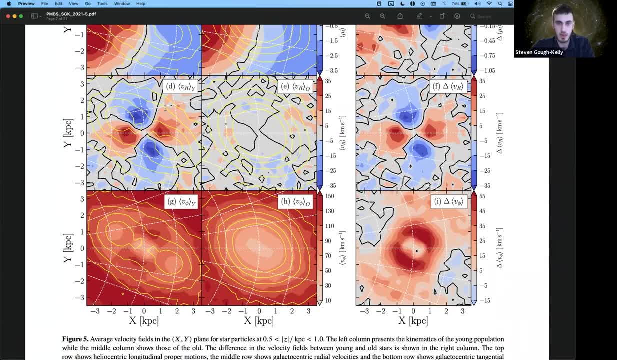 something from my own paper where we can see- I'm using a gas simulation which has which forms stars out of gas. it's not M-body and you can attack. they have cellular ages as well, So you can start to split by different age groups and see what their velocity patterns look like. 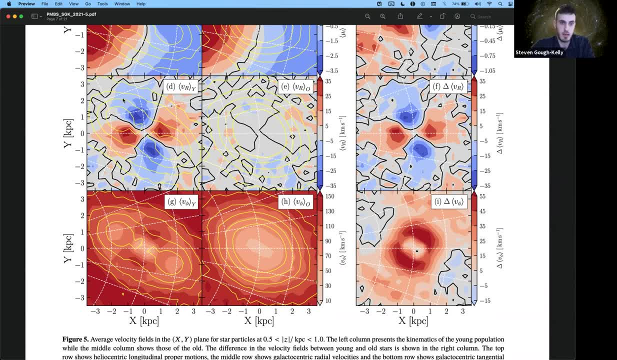 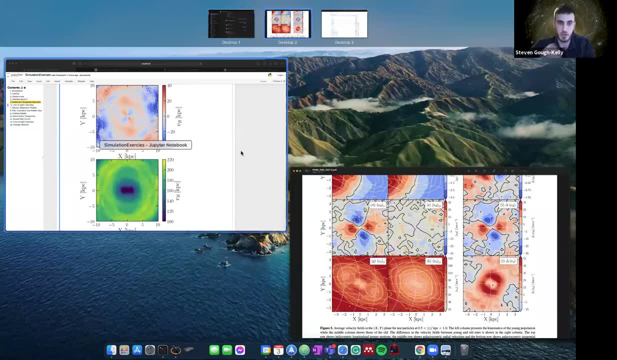 and this is what part of my paper is looking at, And you can see the nice butterfly pattern. the radial velocities is seen in the young stars and not the old stars, So just trying to bring it back into these kind of exercises is something we do in research. quite a 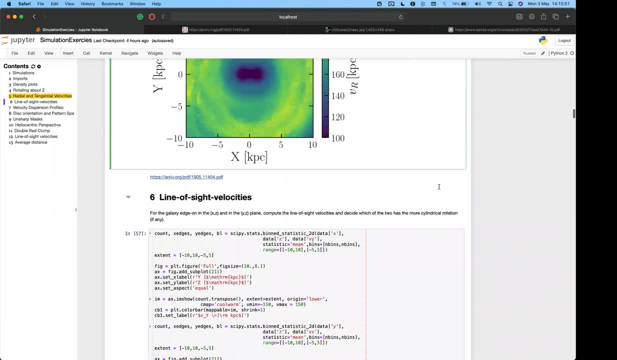 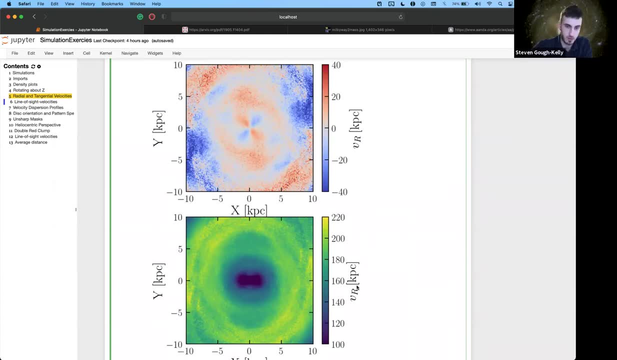 lot. Can I just make one quick comment about the? this is? it's mislabeled. it should be the bottom row. should be V-phi, not V-r. I have missed a V-phi. you're right, sorry, Victor. 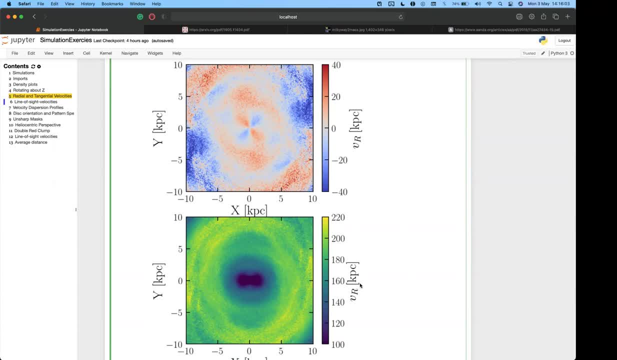 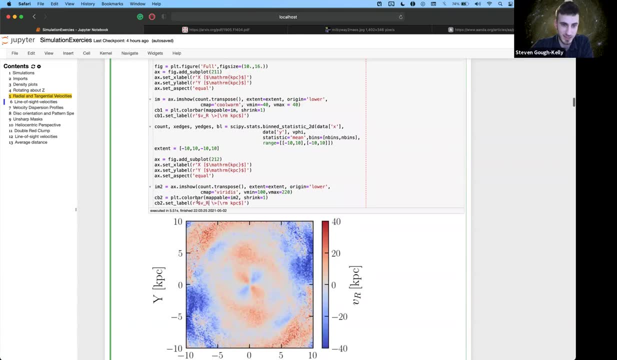 Just in case people. no, it's all right, just in case people are confused. Yeah, sorry, that is V-phi. That's me being a little bit lazy and know that I'm plotting the same thing twice. so I copied and pasted code and I missed my Coulibar label. 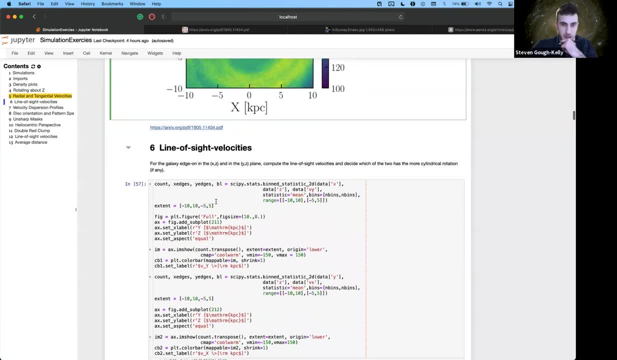 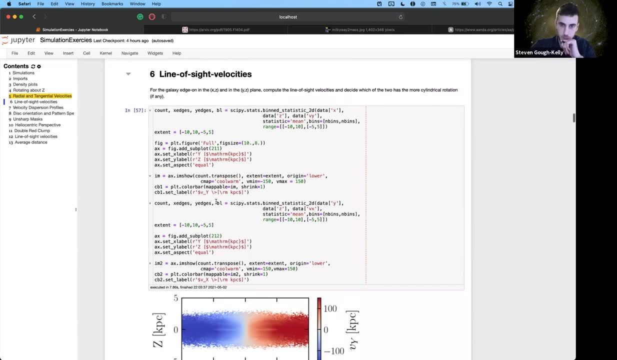 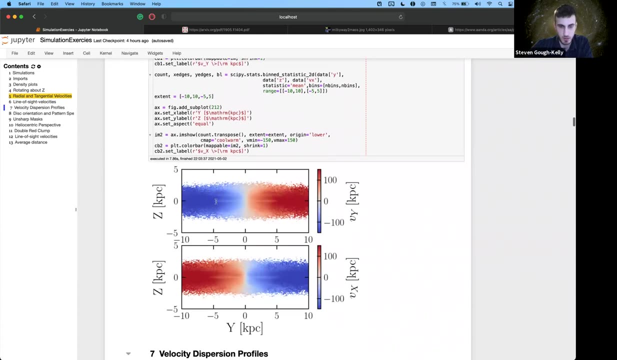 It's V-phi, Apologies about that. So looking into kind of these are kind of line of sight velocities, but not necessarily from kind of a solar perspective. This is just along particular axes. So you've got in a similar kind of way we're looking at. 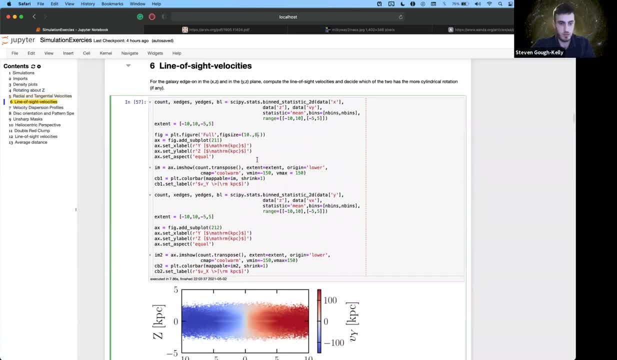 my figures have been too small there, haven't they? Let's see if I can try not to light code too much, but let's see if I can squeeze it in. I'm going to try and get a little bit closer to the top here. 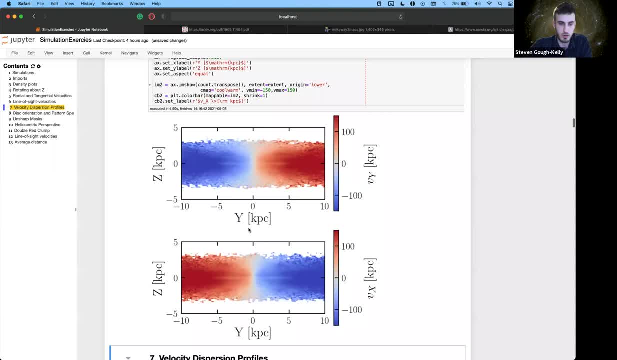 I'm going to try and get a little bit closer to the top here. I'm going to try and get a little bit closer to the top here. Squeeze that down a little bit. There we go. So yeah, Oh, it's both the same axes, anyway. 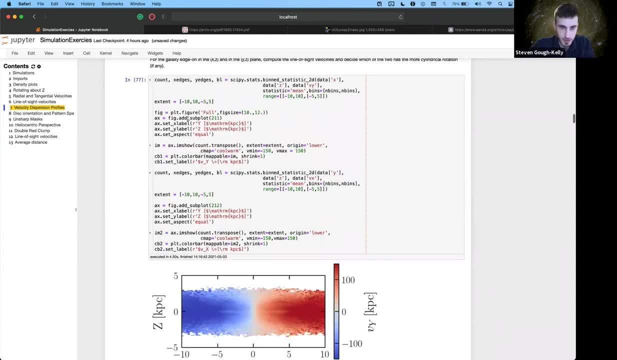 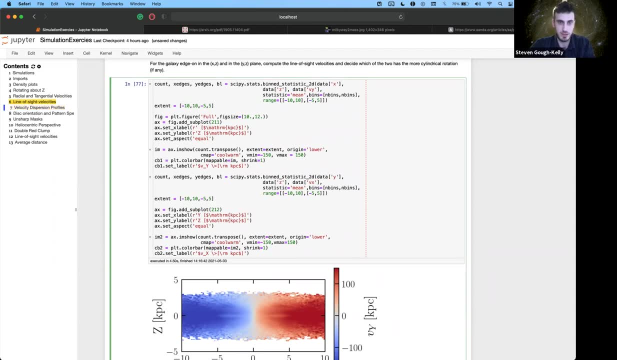 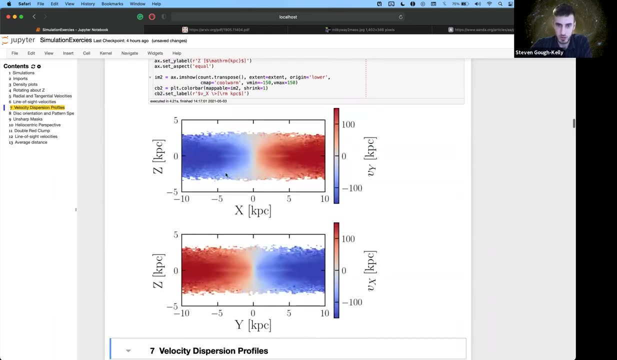 That's great. No, it's not. This is see, you shouldn't light code, but it's got to be done. There we go. We've got the XZ plane, and then the colours is V-Y. and then we've got the YZ plane, we're colouring by V-X, So the 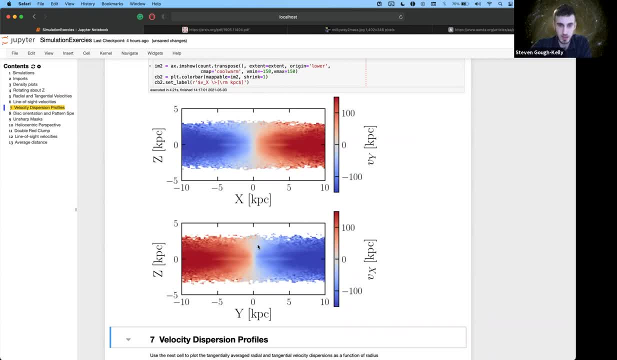 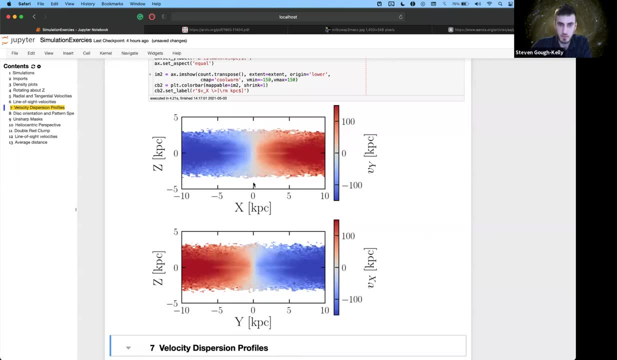 the perpendicular axes to the two that we're plotting here And you can see for rotational systems you get low line of sight velocities near the galactic centre because you're averaging from the near and the far side And then as you move out you're moving through different. the weighting from near to far changes, so you get. 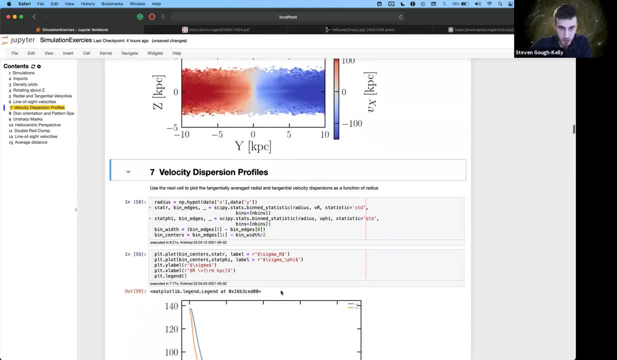 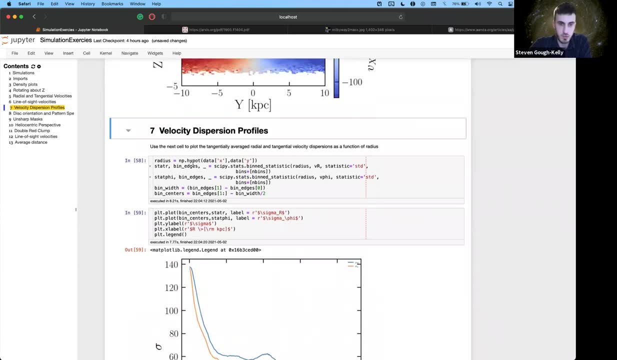 these positive and negative values Moving swiftly into kind of just very simple profiles. You can define a radius within kind of the XY plane by using, like, the hypotenuse of the X positions and the Y positions. You get a radius and then, instead of using 2D bin statistic, I'm 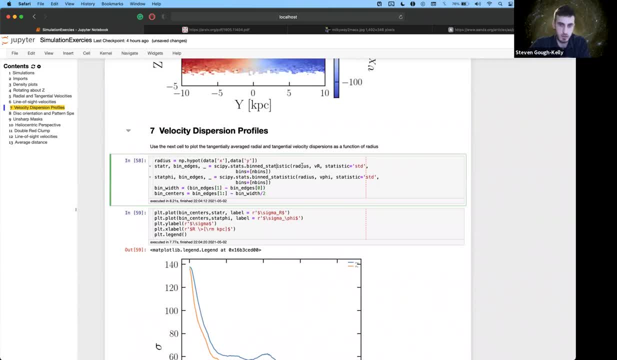 just using the 1D version of bin statistic and we're- excuse me sorry, we're binning in radius and we're binning the V-R and V-Phi values, But the statistic we're using is the standard deviation in each of these bins and then we're plotting just the bin and the standard deviation within. 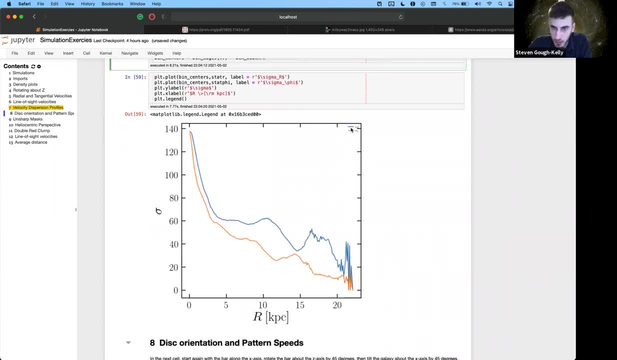 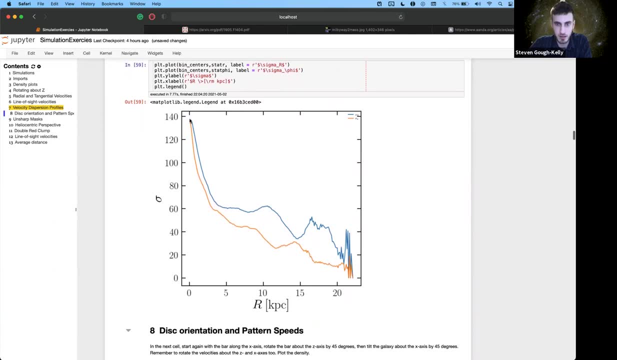 each bin for both of these quantities. I don't know why the legend value has gone so tiny over there, but it has. But we can see just about that. the sigma-R, so the radial velocity dispersion is slightly larger, or radiuses, compared to the V-Phi. Like this is all going out to quite. 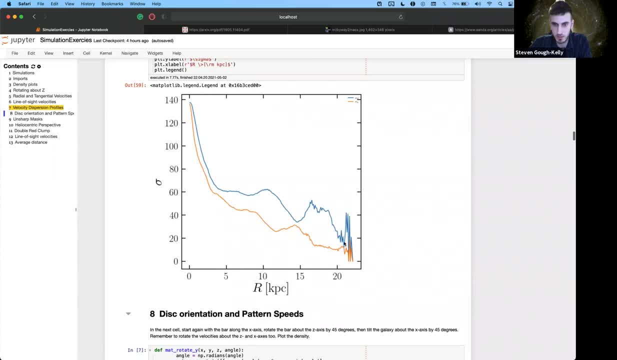 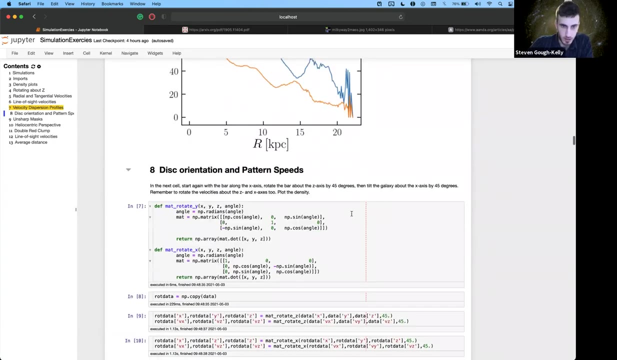 extreme radiuses. we probably won't want to worry too much about here because out here there's so few particles. you can see the actual statistic is going a bit noisy, so we could probably chop that off a bit further in. So we're going to look very briefly at some more kind of orientations and 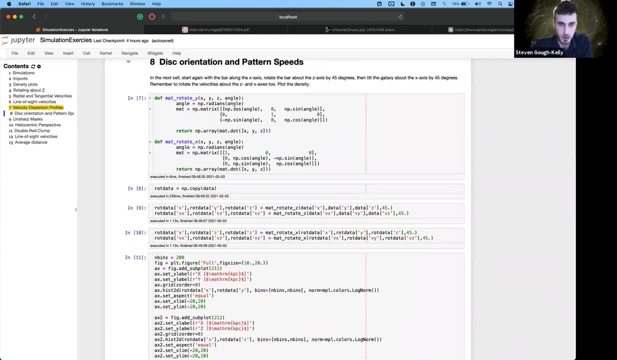 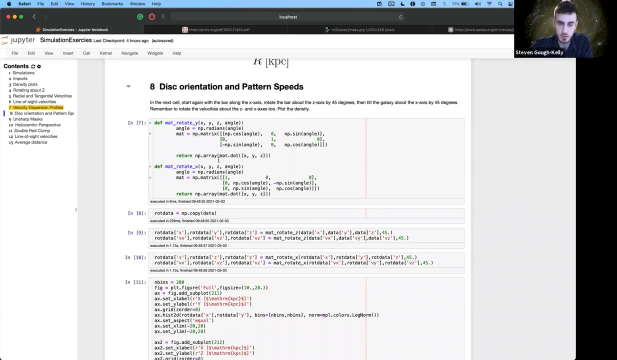 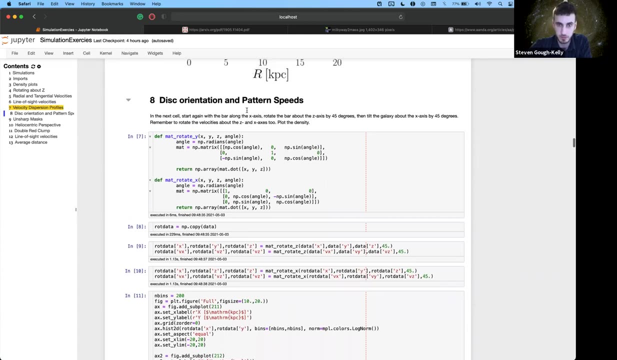 transformations. So I've defined two other kind of matrix rotations in the x and y. I'm only using z and x, but I just defined the y there because it's just easy. I've got all three. now I can reorientate this disc kind of however I want. So we're going to do an orientation in the z-axis. 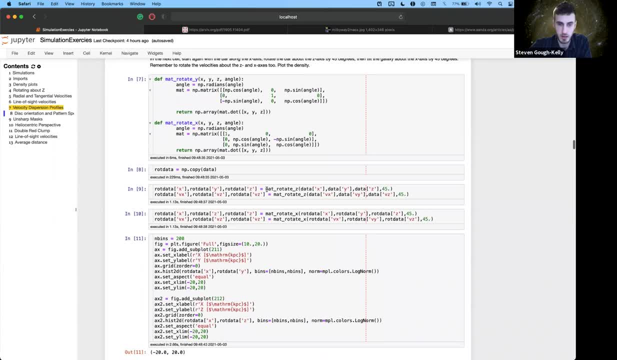 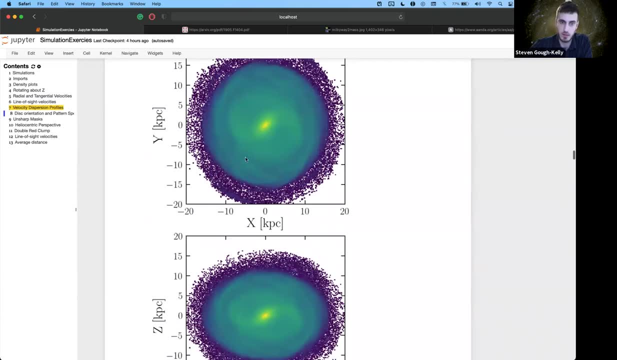 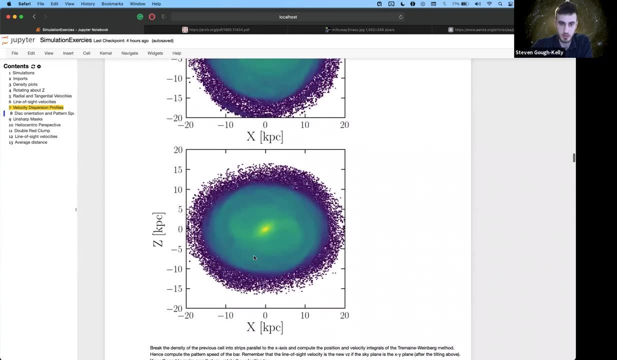 to make the bar angle 45 degrees and then we're going to incline the disc to 45 degrees as well. So these panels show that here you've got the bar. now is an xy now sitting 45 degrees off from the x-axis, and we're also going to incline the disc. so when we look in the x and z plane, we're not seeing. 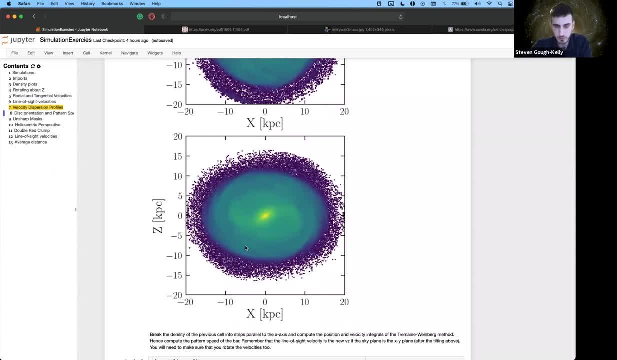 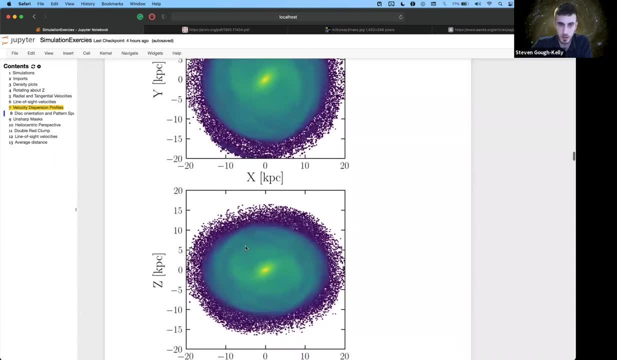 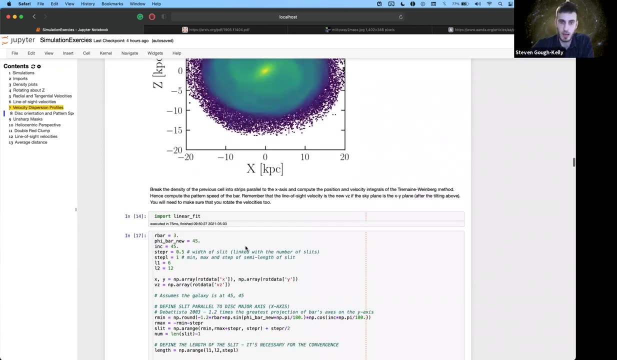 a perfectly fast disc anymore. we're seeing an inclined disc. Now, why would we do this? Well, the exercise: we're looking for the pattern speed of the bar, so how fast it's rotating, and one of the methods of doing this is the tremendous Weinberg method, and to do that we need to know, we need to have the bar, the galaxy, inclined. 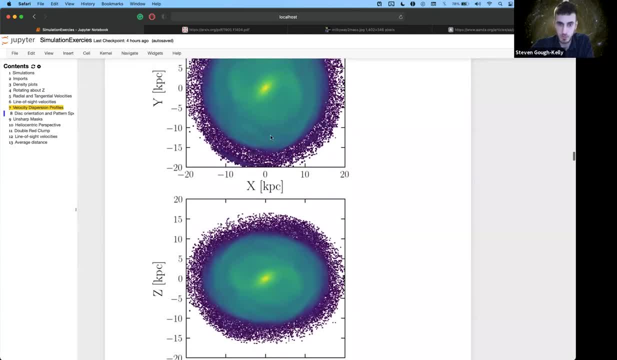 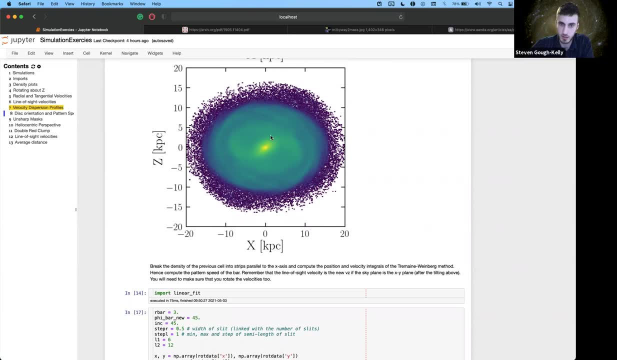 and the bar inclined by a known value. so observationally, you'd have to kind of figure that out for yourself, trying fitting ellipses and such to be able to find those two values. but within simulations we can. we can give it a known value and work from there. 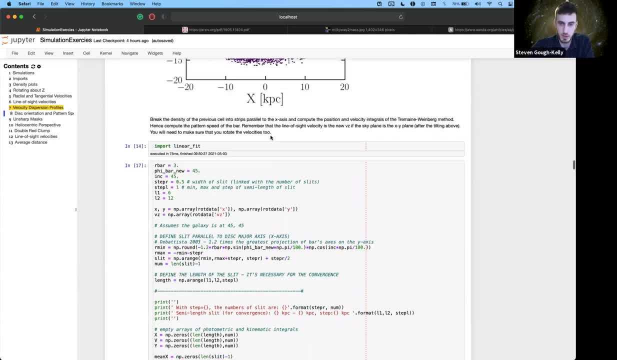 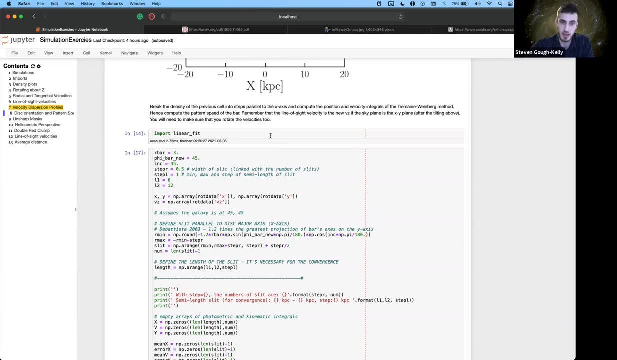 This is a fairly bit of a bit more complex code. I'm not going to go into too much of the details one because I didn't write all of this code. I'm going to shamefully say that I have worked with one of our other students who developed more of this code than I did, but I've been through it and understand its fundamentals. 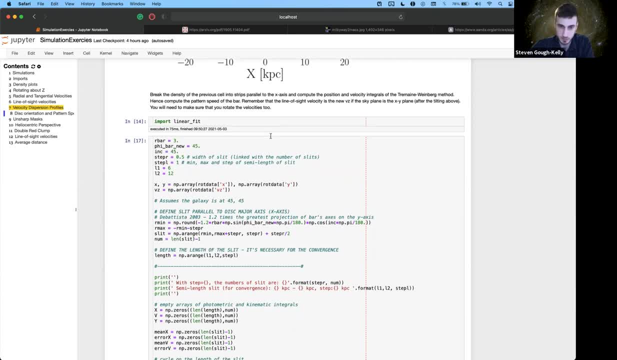 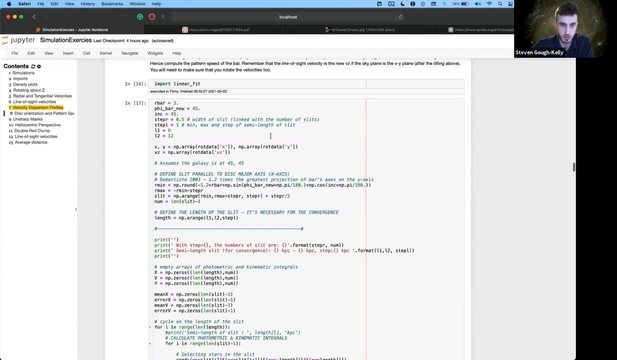 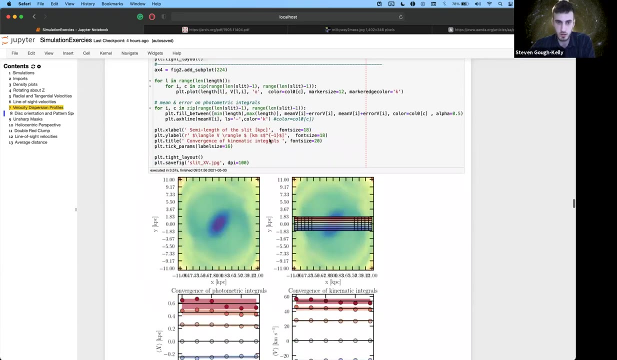 I just didn't spend all the time optimizing it myself, but Chiara, a fellow PhD student, has been incredible working on this to make this code work quite nicely, But effectively we're giving it a. let me show you this figure here: we've got the galaxy inclined and the bar inclined and we're defining slits along the bar. 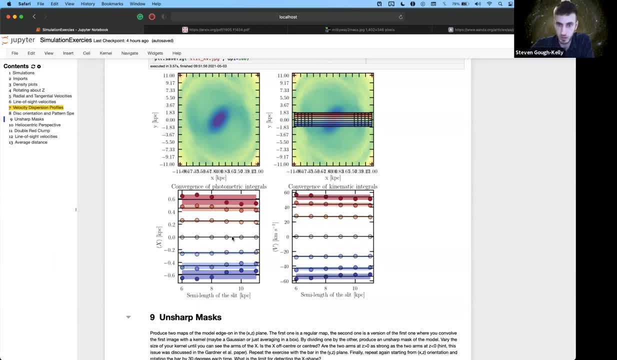 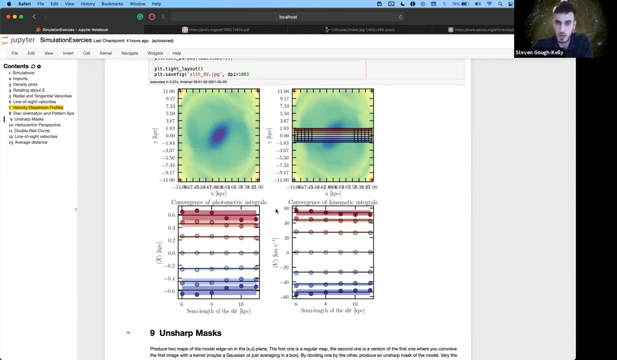 And we're measuring the average positions and velocities and in this kind of scenario, where we're above the galaxy, the VZ component is the line of sight velocity. So that's the component of velocity we using To do this measurement And then, following the paper, that was, 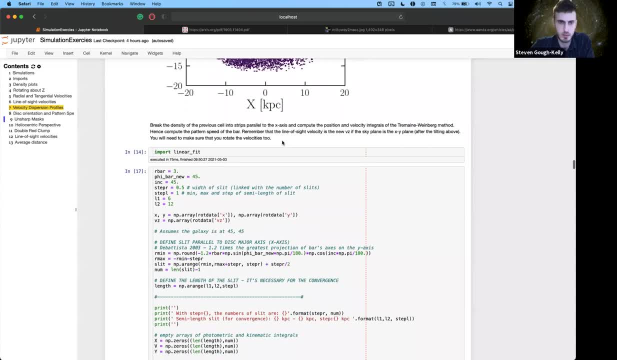 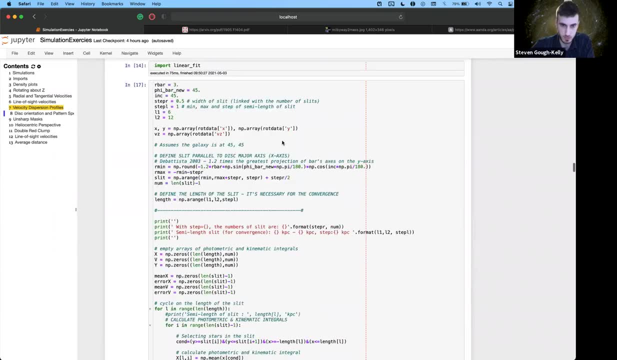 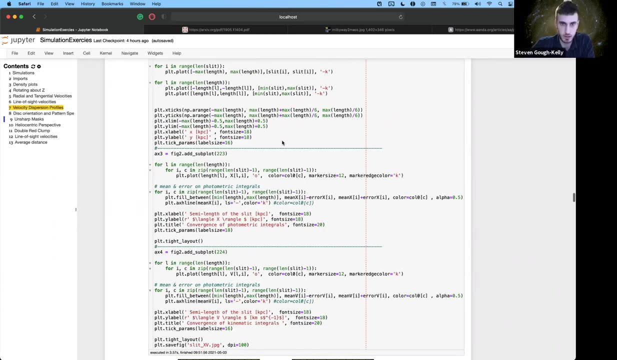 mentioned in the was mentioned in the exercise, wasn't it? Or do you think I've lost the paper, the reference paper for this? I didn't include it, Apologies. I'll find that link for you momentarily, But once you look at these slits and find, 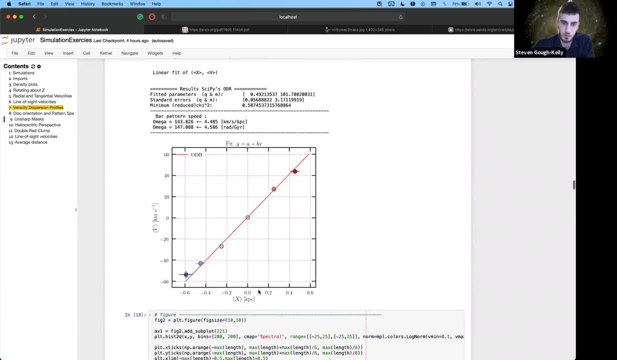 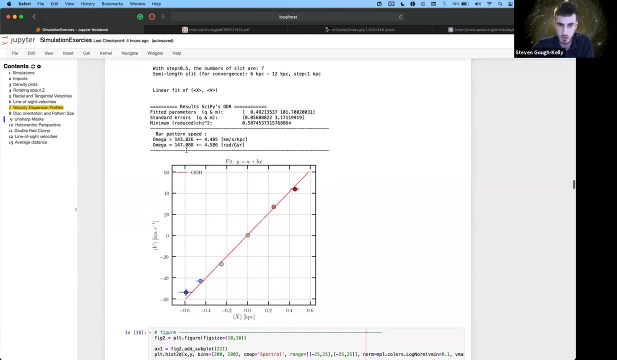 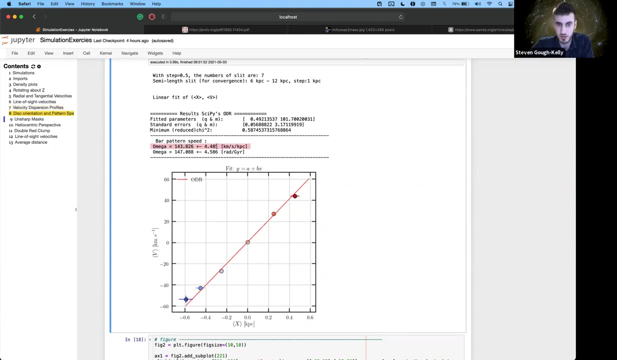 the average positions and the velocities and you put those together, you form a nice straight line and the gradient of this line gives you the pattern space. So for this galaxy we've got a value here: 143, 144 ish, plus or minus five. 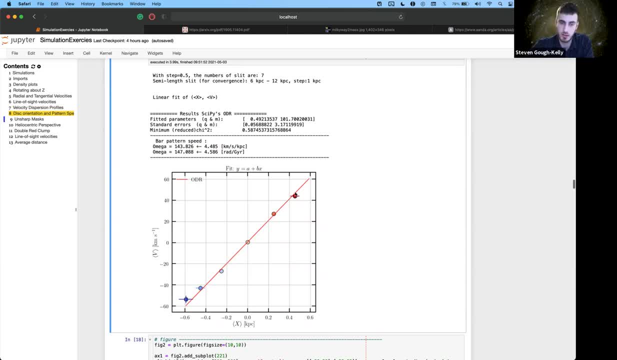 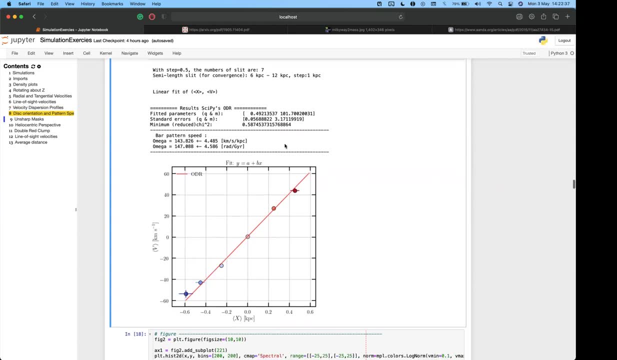 kilometres per second, per kiloparsec. That comes from the gradient and then from some of level of fitting. you can estimate the uncertainty of these kind of measurements And knowing the pattern speed is quite important for studying kind of the bar dynamics. It 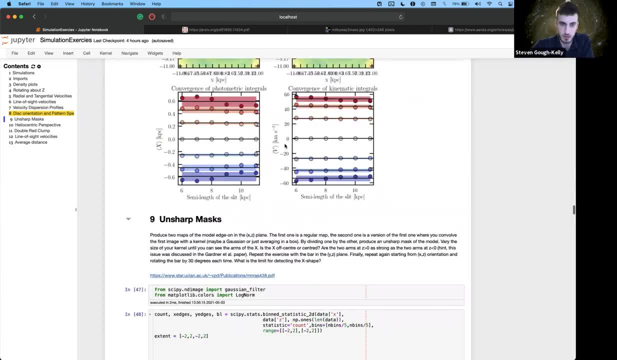 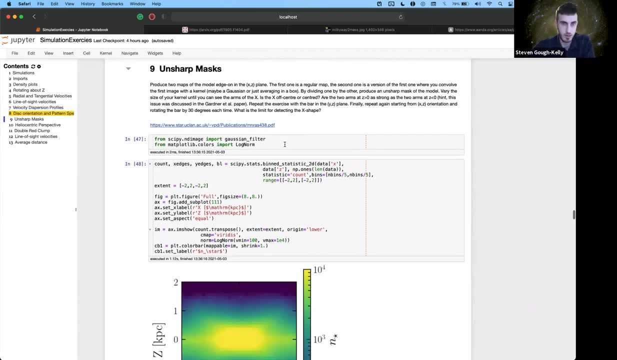 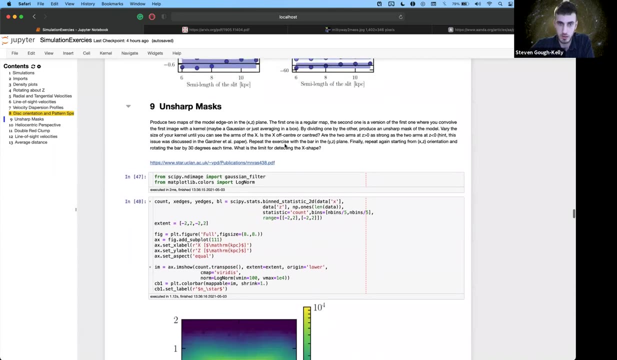 tells you a lot about its resonances and how it's interacting with the disk. So I'm going to move through quickly, So going to start looking at kind of one shot masking something that the observation is to a bit of a different level of accuracy. So I'm going to import a few more. 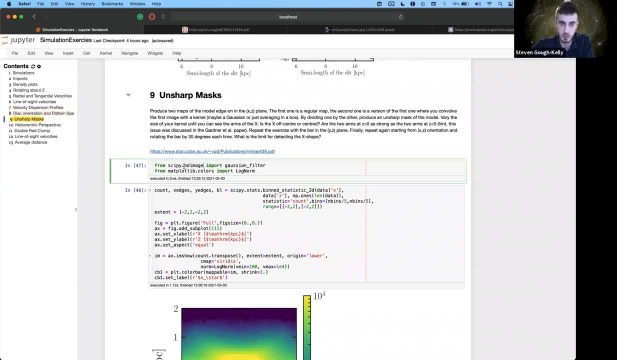 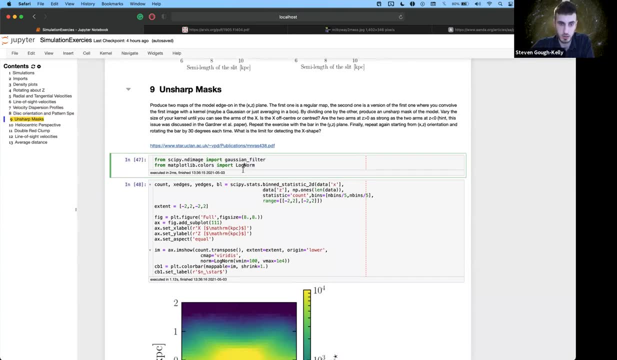 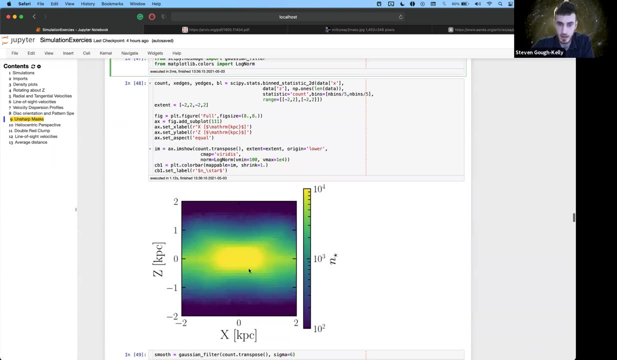 libraries as well. some more modules from libraries have already imported sci fi, but I'm using importing a Gaussian filter And from app live I'm using just a log norm just to help with plotting. So we've got back to doing some normal exit. 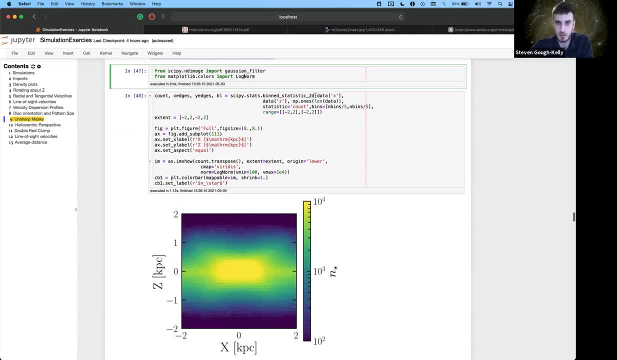 density maps and using in statistic 2d, So the third axis, instead of using kind of velocity or anything like that, I'm just producing an array of one values- the length of the actual number of particles I've got, and then using the 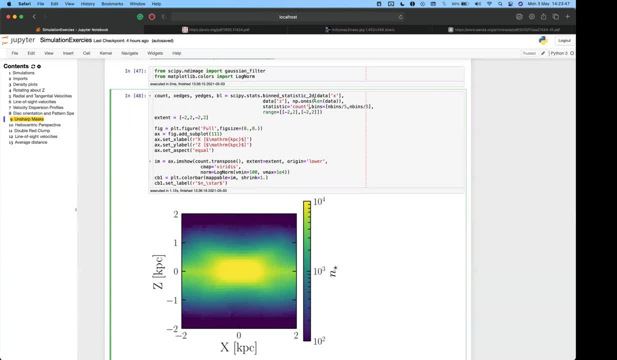 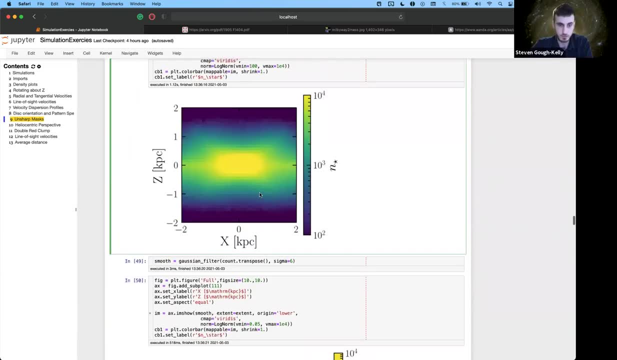 counts statistics. So this is the sum of the data points in each in each 2d bin. So that's what we get, And same as before, I'm just a bit more zoomed in. Well then, what we're going to. 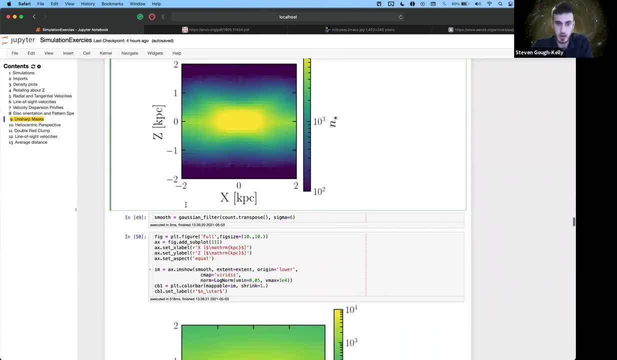 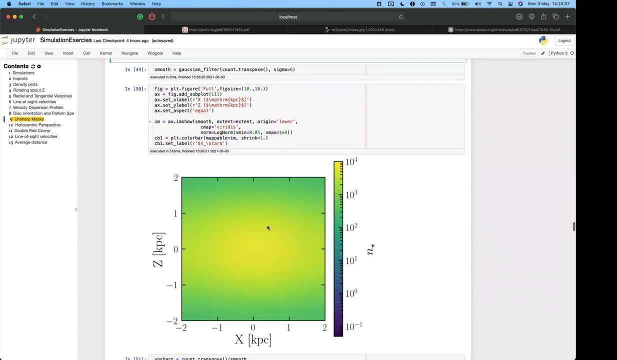 do is we're going to take this image and we're going to smooth it with a Gaussian filter, Relatively high sigma, so it's going to be quite smooth, And what you end up with this after you've smoothed it, which is just kind of the 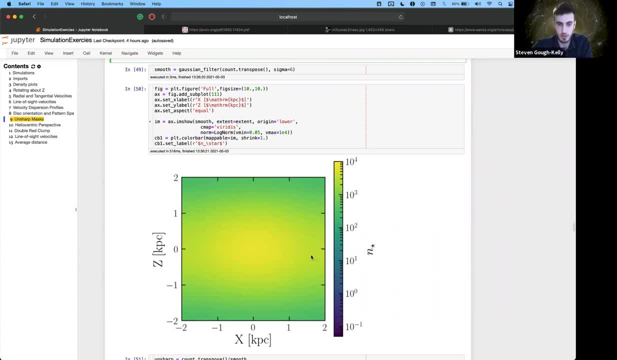 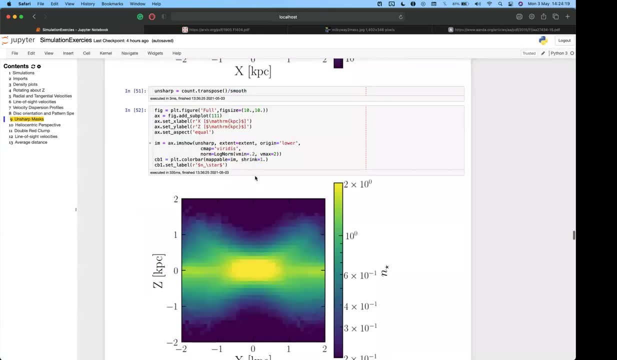 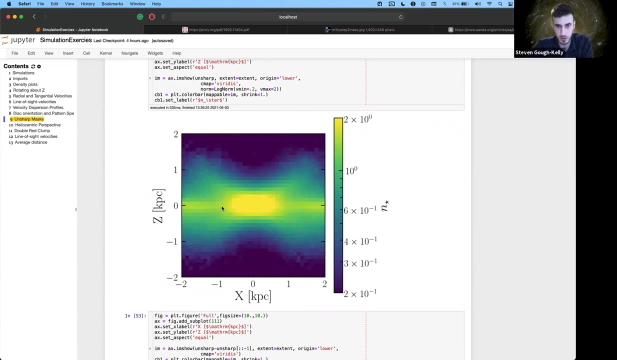 average kind of density in x, z space, And then we do the original image, divided by a smooth image which leaves us with this, which is an unsharp mask, And what you can hopefully see is that the kind of the kind of non-axisymmetric. 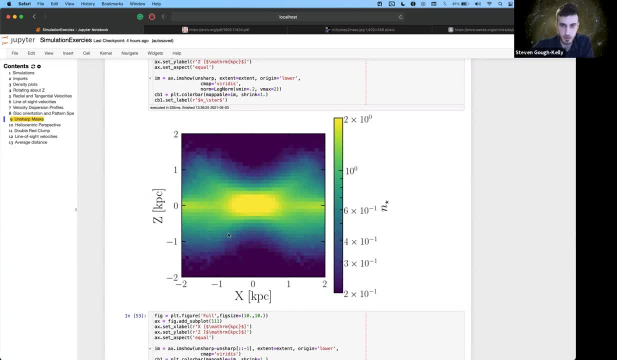 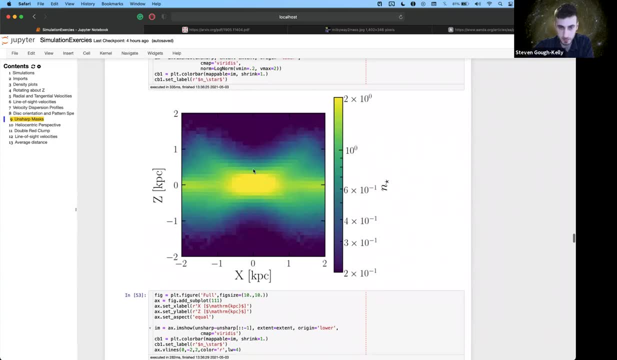 features or the kind of the, the kind of unsmooth features, are pulled out a little bit more. they start to be a bit more defined, And what you'll hopefully notice in this image is that the x shape is not particularly symmetric about the. 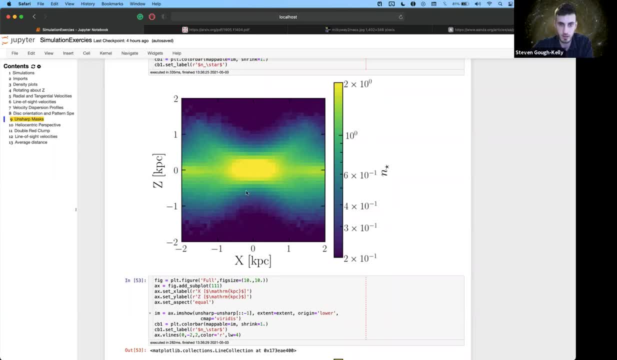 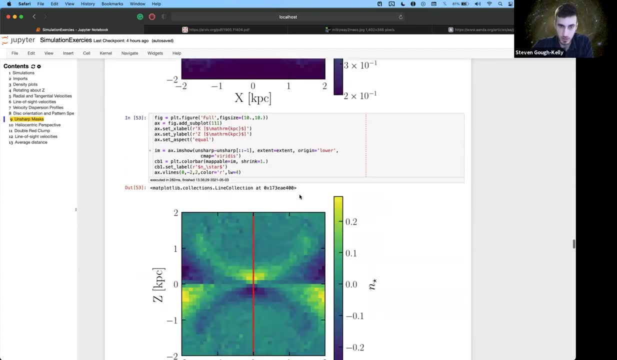 plane about. z equals zero And it's a little bit asymmetric. the top half is slightly larger than the bottom half. To kind of convince you of this, I've just done a very quick difference map, So I've just taken the unsharp image minus. 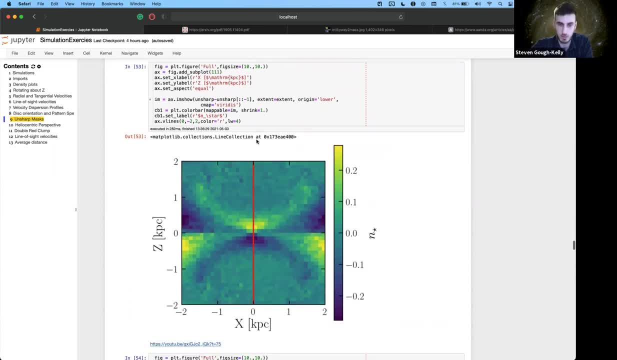 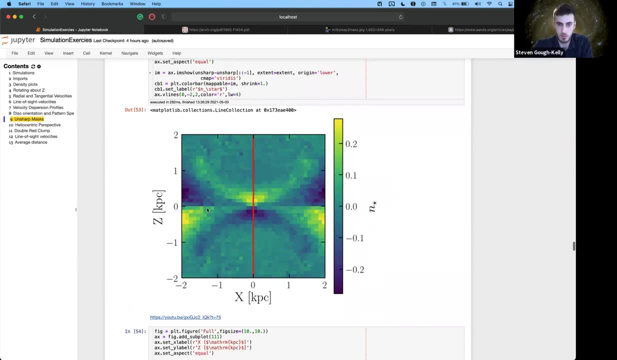 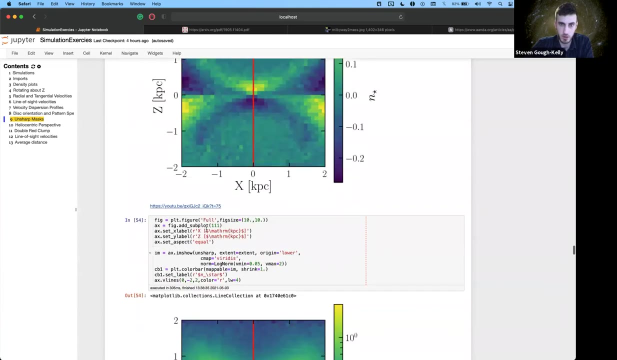 the unsharp image flipped about. the flipped about one axis, So the y axis is flipped And you can still see this differences from above and below the plane. Now, this is kind of what we expect for the kind of evolution that this bar went through. I 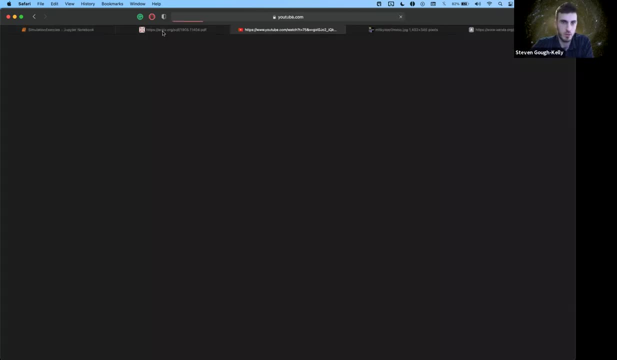 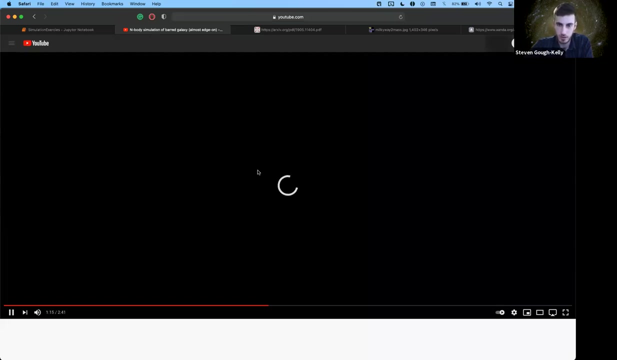 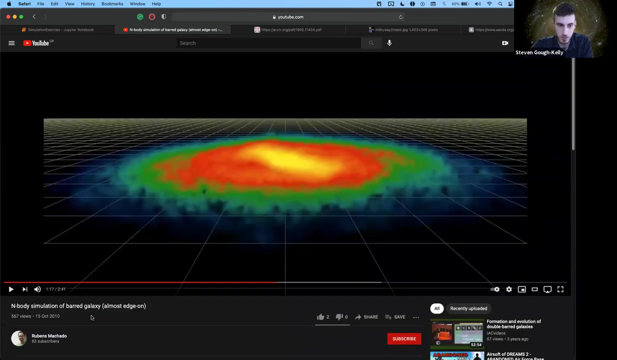 was going to find a gif from my own research, but I found this as well, So hopefully my connection stays stable enough for this to play. Well, this is an M-body model from Rubens Macchiato. very kindly lets me share these. 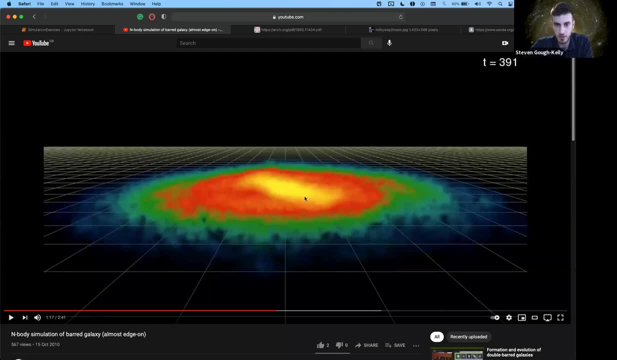 videos, And what you'll see is this has got a very strong bar. this is slightly- slightly in the x-head plane, but it's just slightly above it, So we can see some of the disc as well, And it's got a very strong bar. And what's about to happen is that. 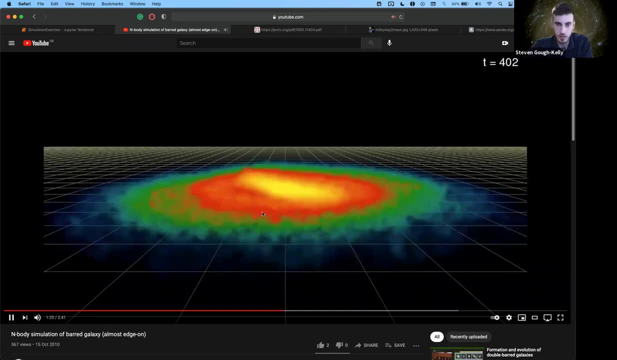 the bar is about to buckle And what you'll see, hopefully, is that, as the bar starts to bend, let me see if we can get a nice orientation here. you see that the bar is buckled and bent and you're starting to produce this x-shaped feature. What you can 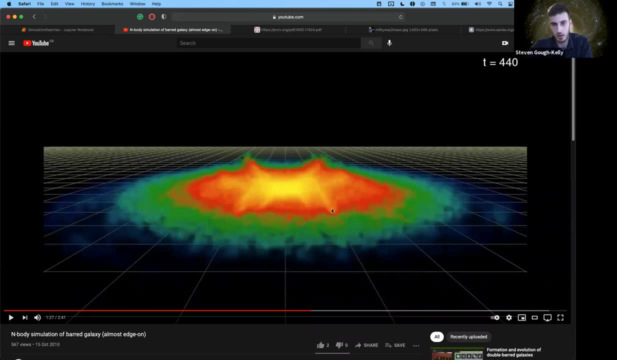 see, hopefully- is that the arms below the plane here are slightly larger than the ones above the plane. So this is the buckling instability within bars And this is how one of the mechanisms that galaxies can form these x-shaped kind of structures, and R1 went through. 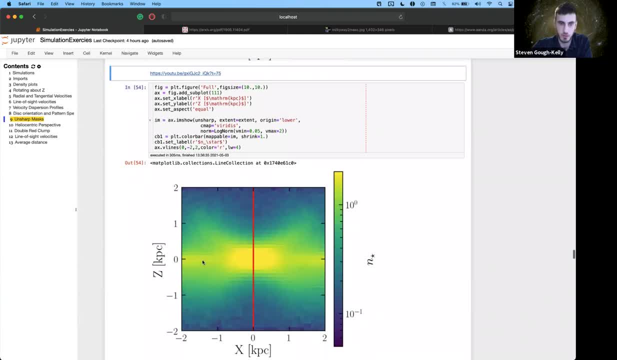 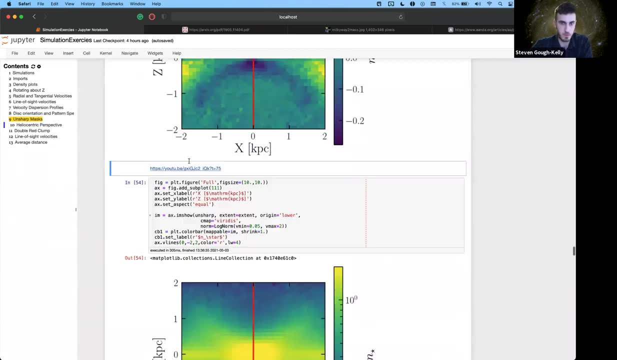 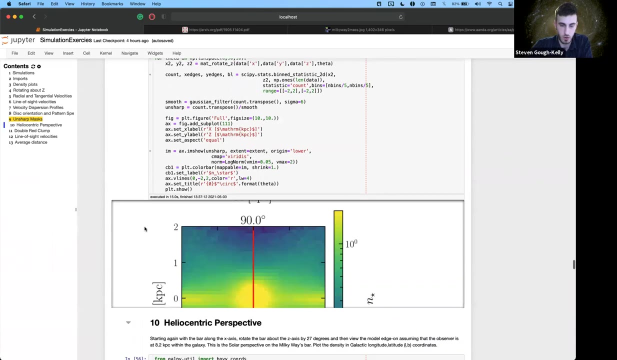 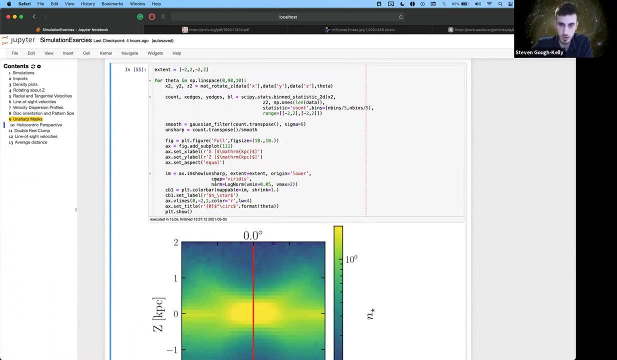 this kind of buckling, instability and formed this kind of asymmetry above and below the plane. So as we kind of finish in touch with this exercise, this one we were looking at- we're interested to see kind of what orientation angle this is going to be. Can you see the box peanut still? So I'm 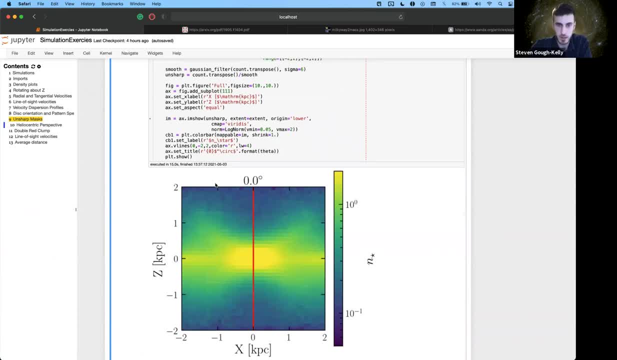 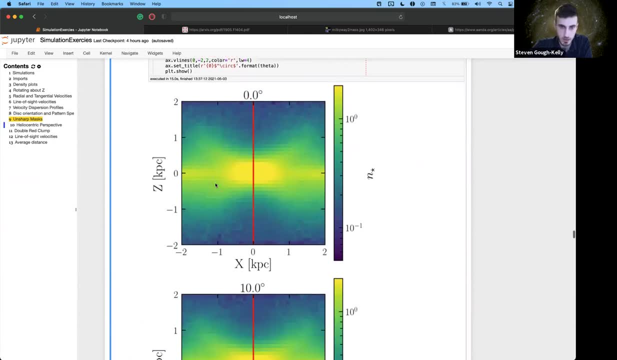 going to use the unsharp mask because that seems to be the best method of kind of detecting the x-shape and the clearest image of it, And I'm going to step through different degrees of rotating the galaxy about the z-axis. And, for the majority, 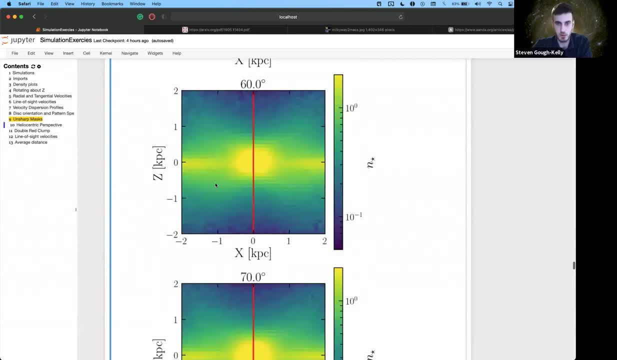 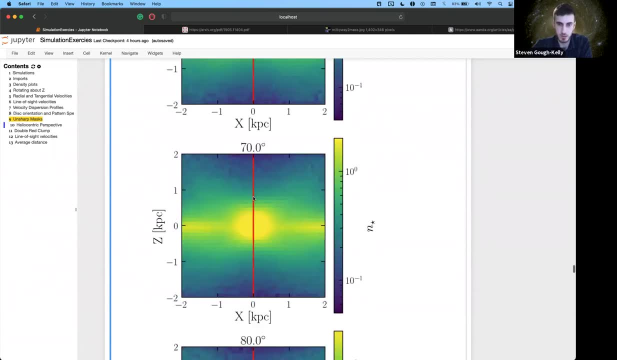 whoops of the rotations. we can still start to see it At 60 degrees. you're still starting to see some. At about 70 degrees. we're starting to lose it, And then by 80 and 90 degrees with the bar. 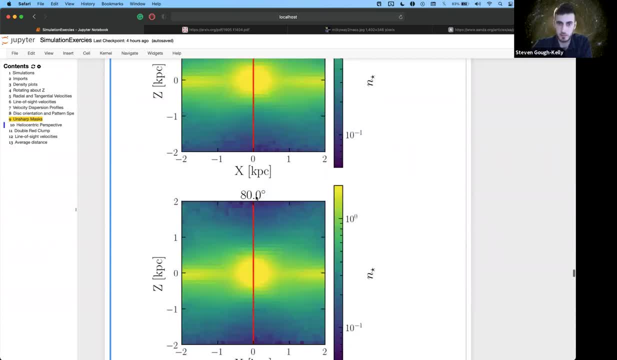 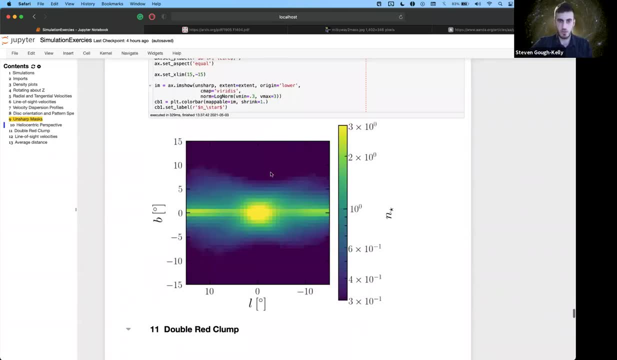 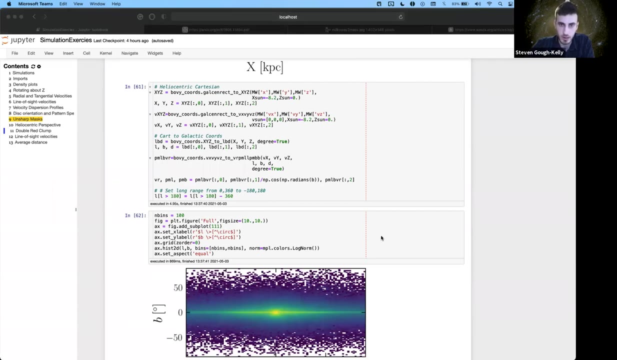 seen end on. we're no longer seeing the x-shape. So, following on from this, we've done a lot of things. Apologies, That's my team's going on. We've done a lot of things from kind of Cartesian coordinates. 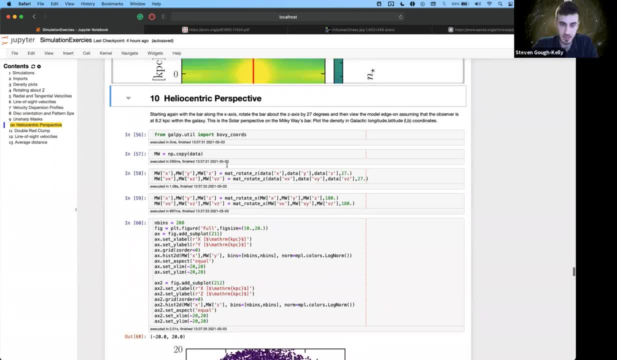 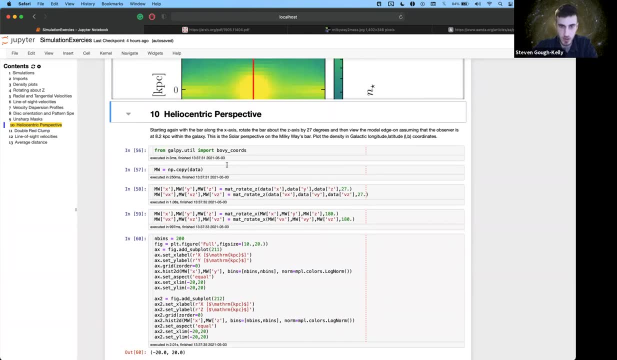 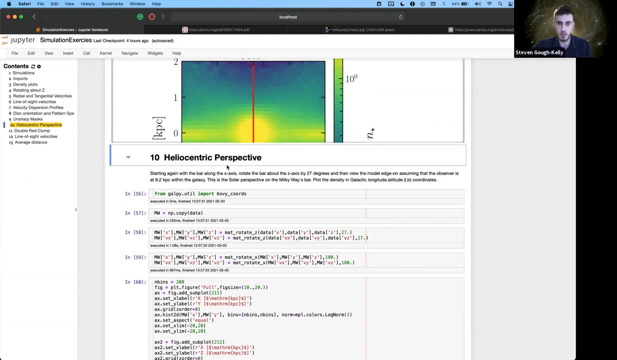 looking in x, y, z space. Obviously this isn't how we observe the Milky Way. We're sat inside the Milky Way, We can't manipulate it in this kind of way And so we have to use. we're stuck with kind of more, with a coordinate system from 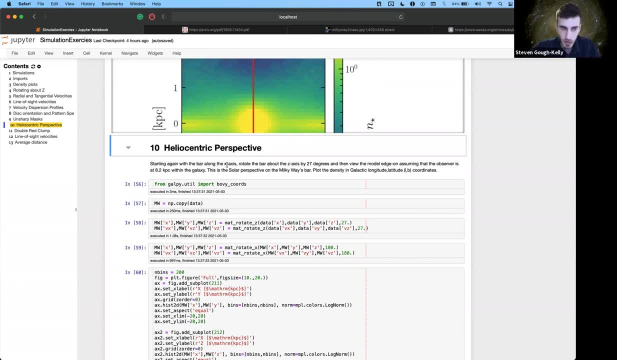 the observables really Our world is in. we perceive kind of the universe out from our viewpoint in kind of angular coordinates and our angular perspective. That's how we basically measure things through telescopes. So when we're trying to do comparisons between our theory and Milky Way observations, we 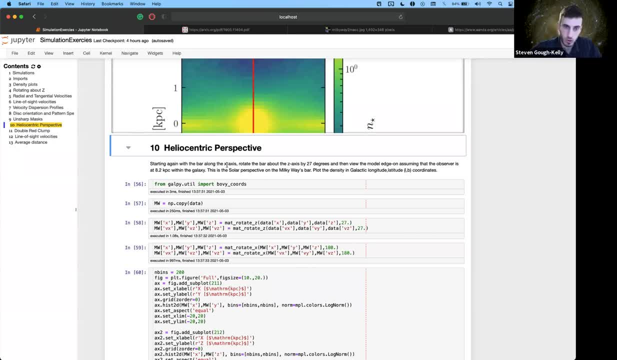 kind of have to find some common ground So we can look at our simulations from kind of the solar perspective. we can approximate that You can do these coordinate transforms through equations and following the mass through. It's probably a bit too convoluted and 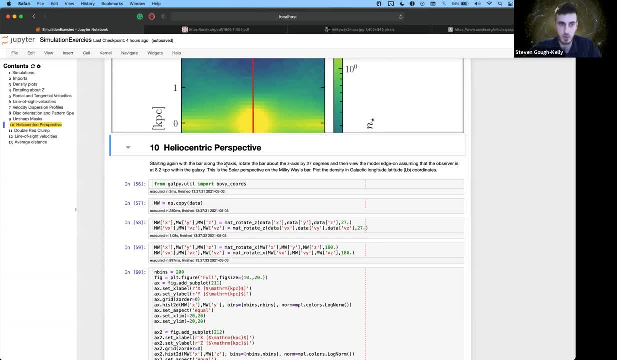 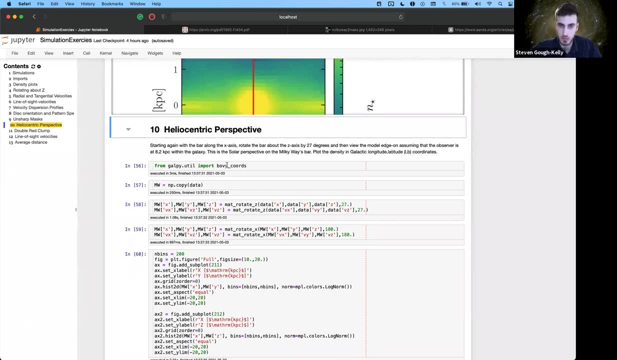 long winded to go through in this kind of session or speaking for long enough as it is, So I'm just going to use a package- just a sneaky little shortcut- from GalPi which includes some level of coordinates transformations. AstroPi has a similar kind of. 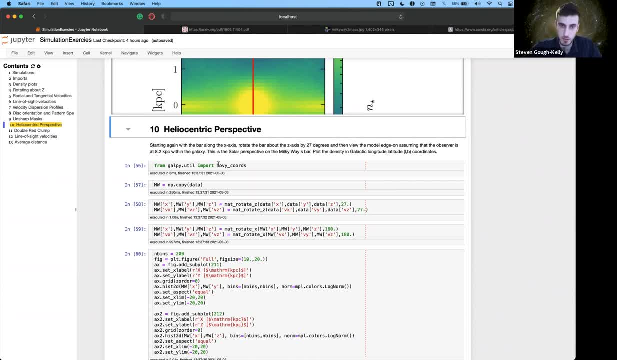 set of functions and coordinates. Again, this is from my work and my research. I've used GalPi for my work, So it's just it was easy to follow similar lines of code. So we're going to try and approximate the Milky Way using the model that we. 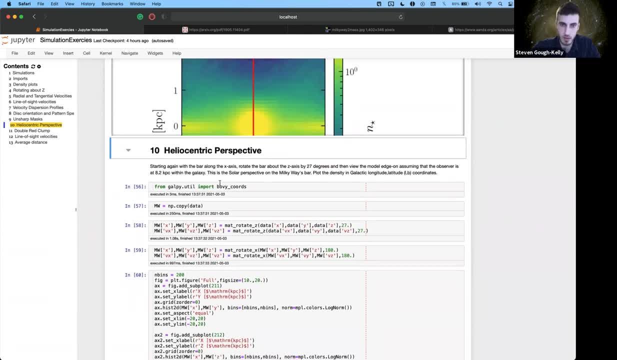 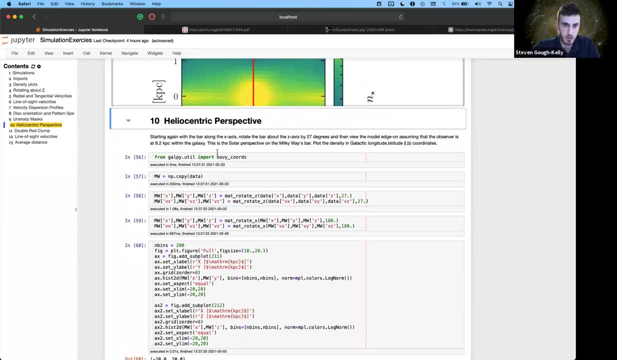 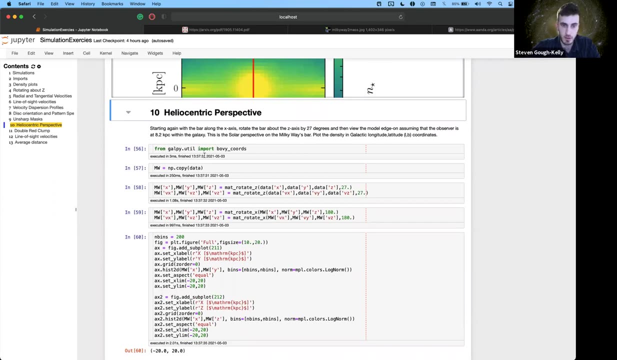 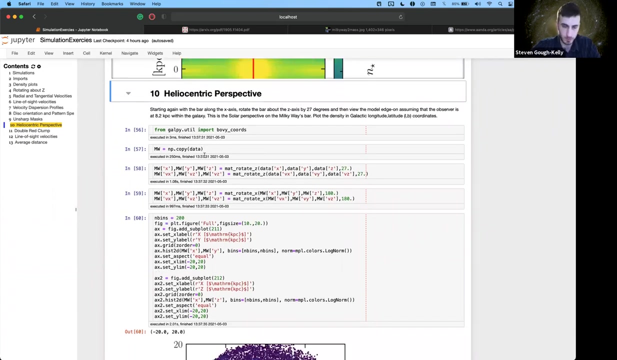 have here. It's already been rescaled to kind of the similar parameters to the Milky Way in size and velocity, I believe. So we're going to just convert directly from the Vx, Vy and Vz into observational coordinates like galactic coordinates. So for starters we're 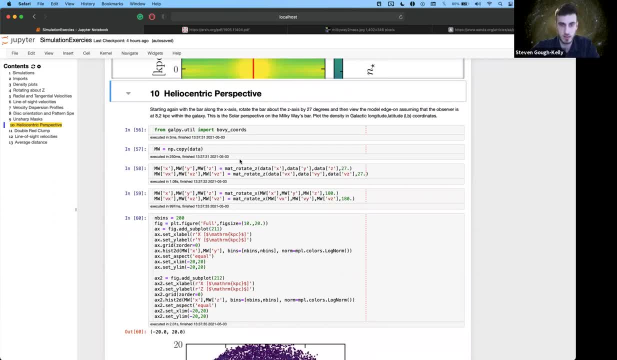 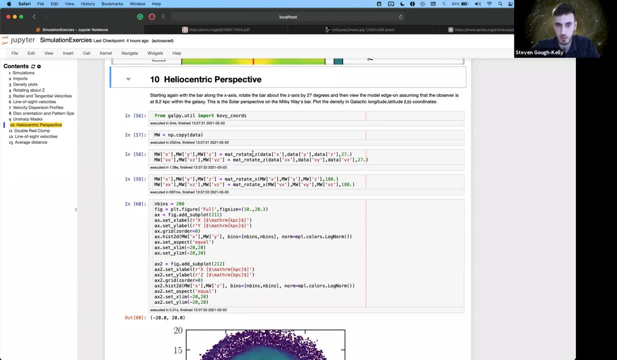 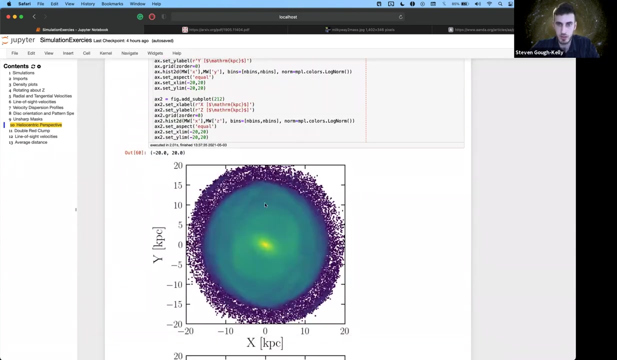 going to take the just kind of the base model with the bar lines along the x axis. We're then going to do a rotation of the bar to the approximate Milky Way bar inclination angle, which is roughly about 27 degrees. And then this rotation, this matrix rotation, goes anti-clockwise. 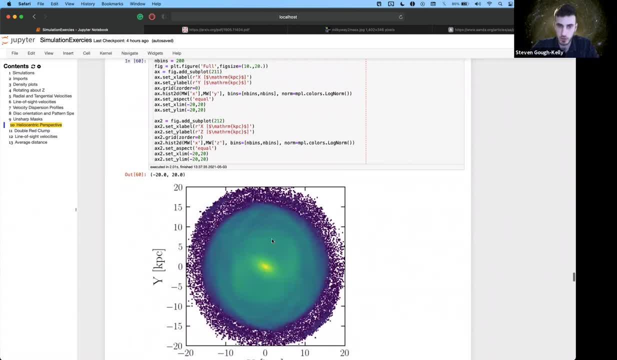 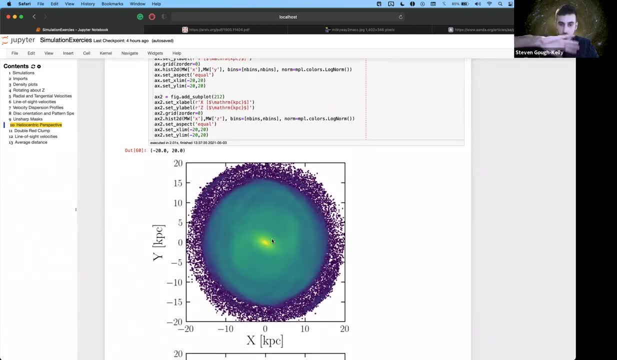 So it will put the bar down here. So all I've done to also flip the velocities in the direction of angular momentum, I've just flipped the entire galaxy 180 degrees face on the other way. So now the bar points up. this way I'm going to place the observer at minus 8x. 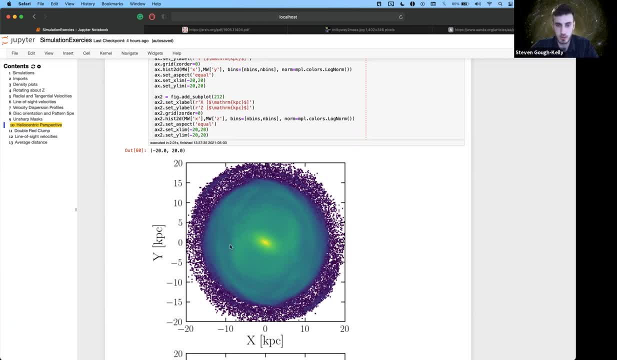 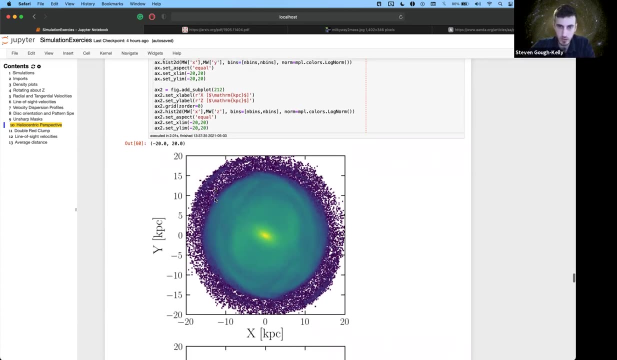 over here, So that when we look at the center of the galaxy- so if the observer is at minus 8 here and we look at the center of the galaxy- the near side of the bar, or the bar that's closest to us, is off at an angle that's off to our left, So the bar points up. 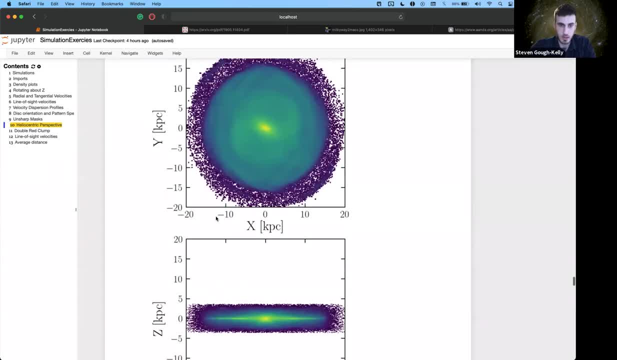 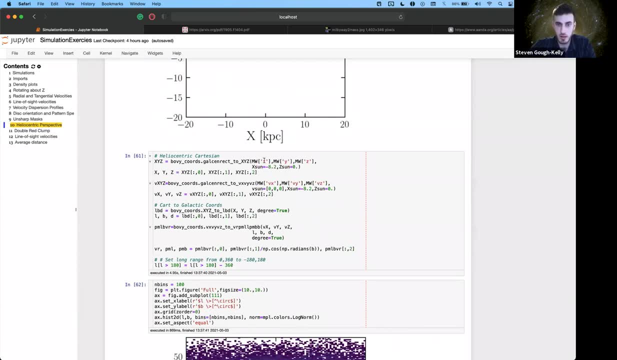 to 2y. So here's the xy projections from there. We're then going to do some coordinate transformations. So we're going to do the galactic-centric xy-projections, We're going to do the galactic-centric xyz, to do a heliocentric xyz. 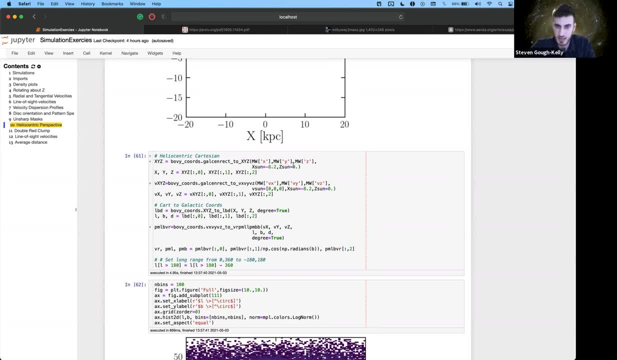 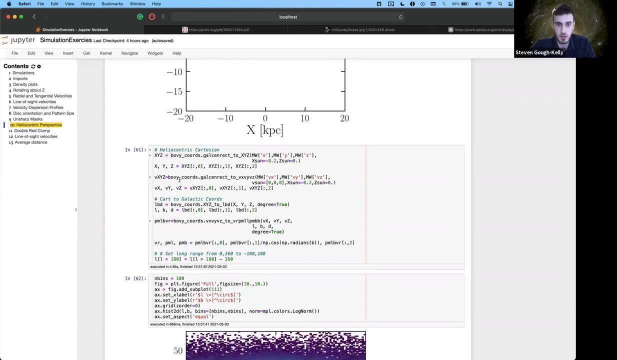 where we place the Sun at minus 8, 8.2x, We're keeping the Sun in the plane. It's kind of slightly out of the plane, but not by enough to worry about in this kind of context. We're then going. 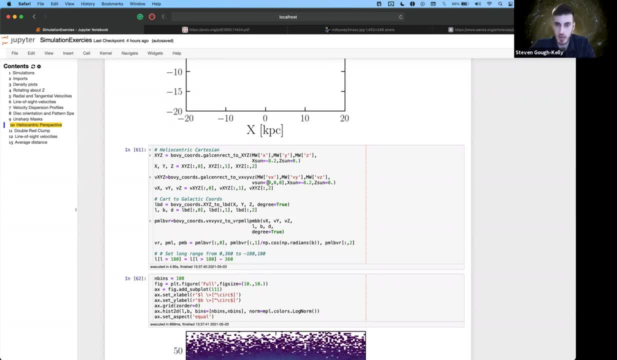 to do the velocities as well. We're going to stay within the galactic rest frame. We're not going to add some velocity to the Sun, because the Sun is obviously moving around the galactic Center, So it has its own inherent velocities that we have to account for. 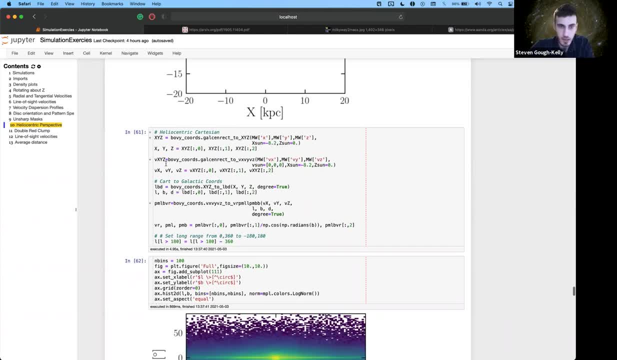 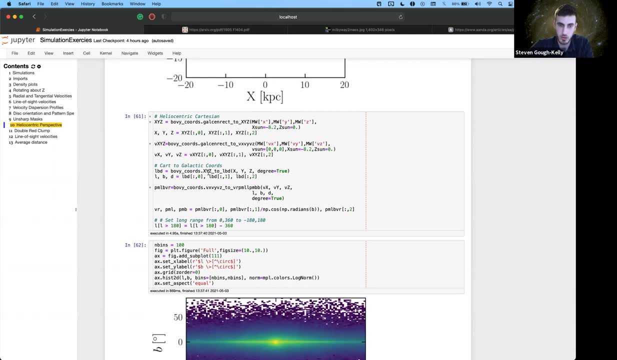 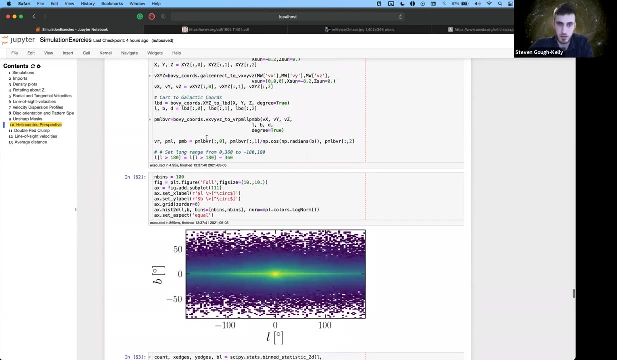 but we're going to stay in the galactic rest frame and then we can kind of put these heliocentric xyz into long-issue latitude and distances from the solar perspective. So that's all that cells are doing. The final step here is the GalPi routines. returns L from 0 to 360.. So all I'm 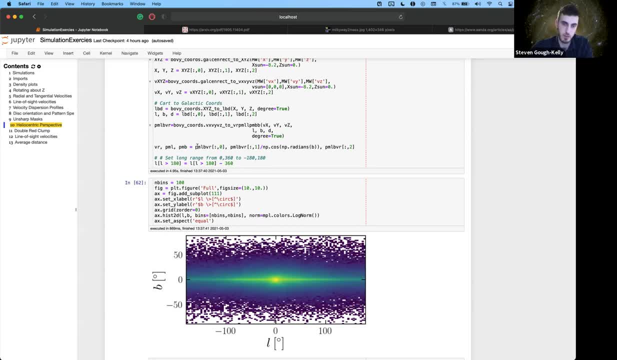 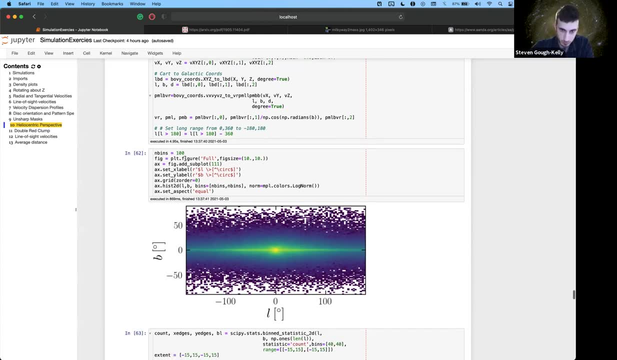 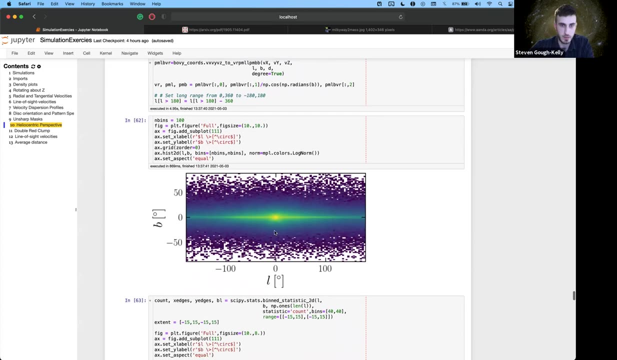 doing is just beyond 180, moving everything back by 360, so we go to minus 80 to 180 as the full range, which is typically more common, because this places the sum at zero degrees longitude. So here is all the data in LB space. You can see 180 in either way. so we've got the galactic. 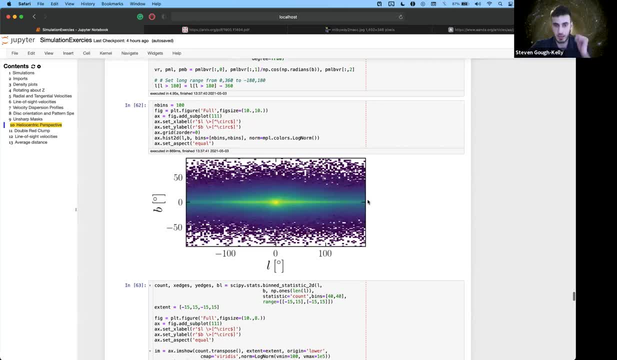 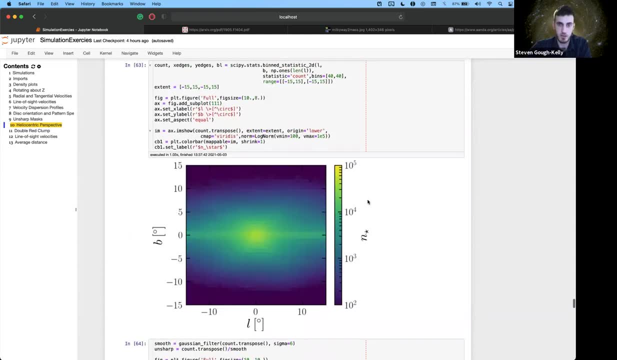 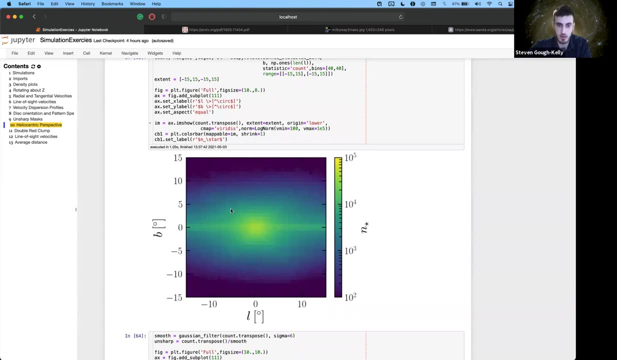 center and then 180 minus 180 would be the galactic anti-center, pointing to the wall. So we restrict ourselves to kind of just a smaller window. if we just look at, say, minus 15 to 15 degrees in L and B, we can start to see the beginnings of 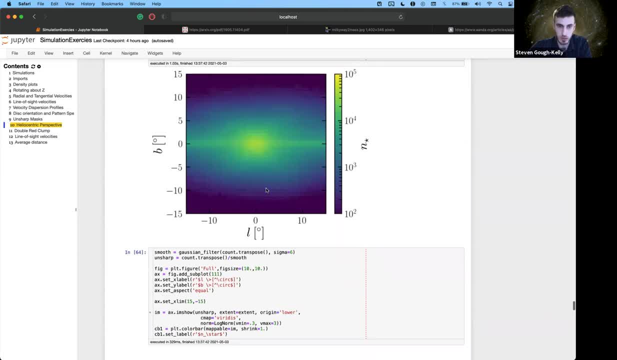 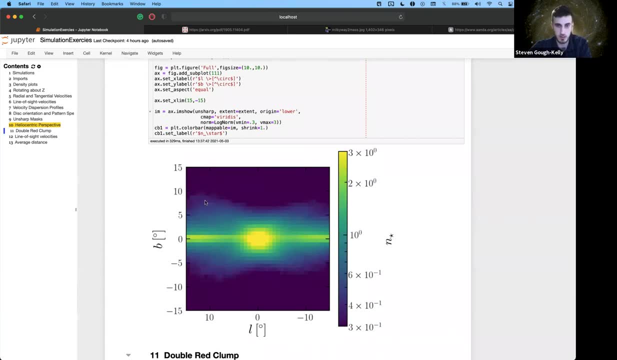 an x-shape coming through. This isn't the most clearest plot. if I do an unsharp mask again, you can start to see an x-shape, but what you'll notice, instead of it being quite a nice, the the arms of the. 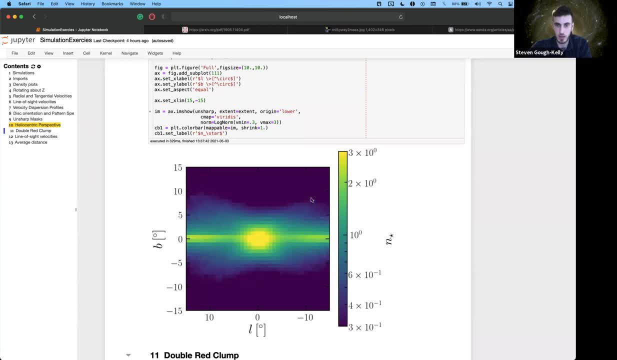 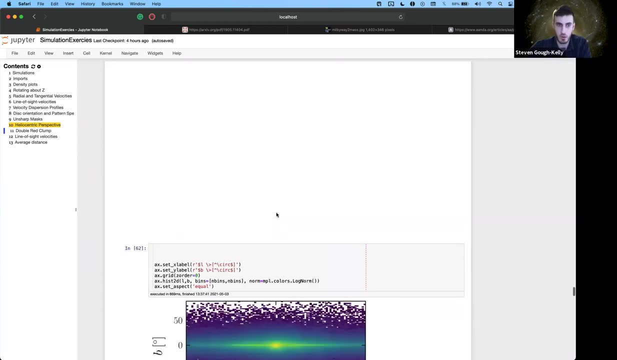 x-shape, at least on one side of the galactic plane, being equal in their height. we've now got one that sticks up a little bit higher on one galactic magnitude, not necessarily on the other, And this is kind of what we were exploring earlier when we were changing the orientation of the disk. 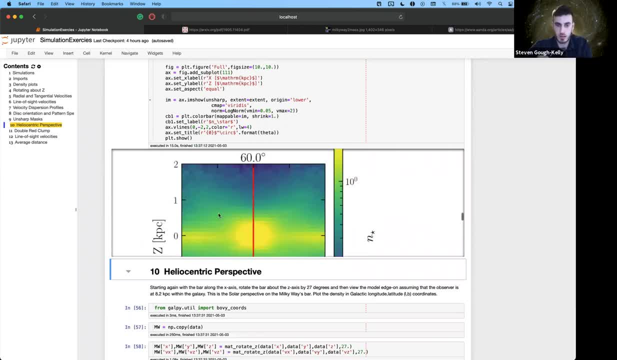 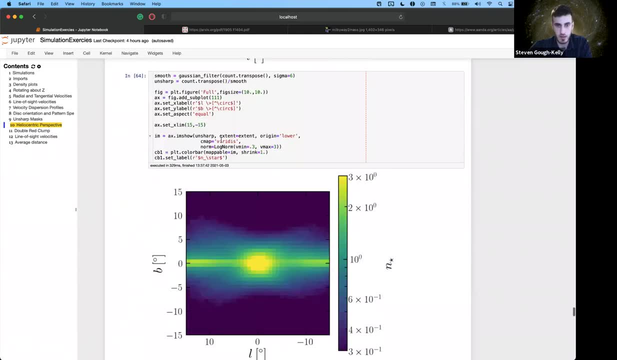 and we were rotating by z, we can see that the arms of the x-shape move. in our view, and because we're now in a kind of an angular coordinate system, the near arm is closer to us, so we actually see it for a larger range of latitude values than the other arm. 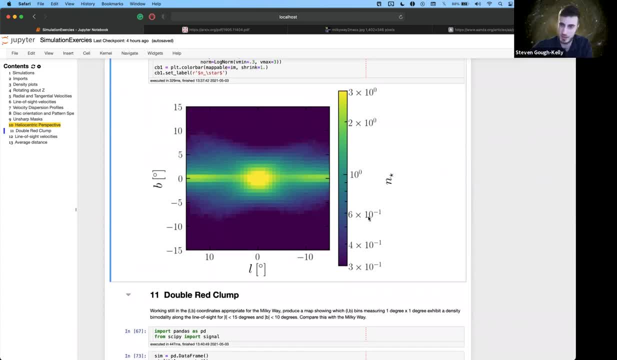 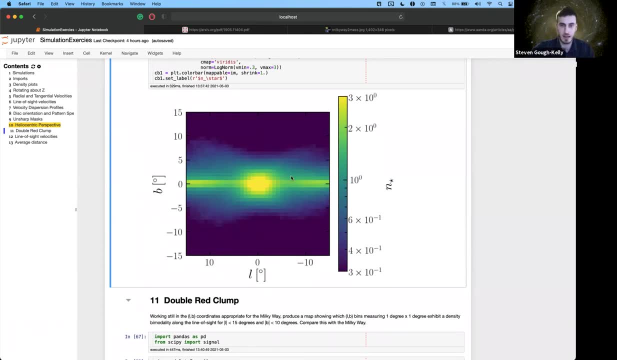 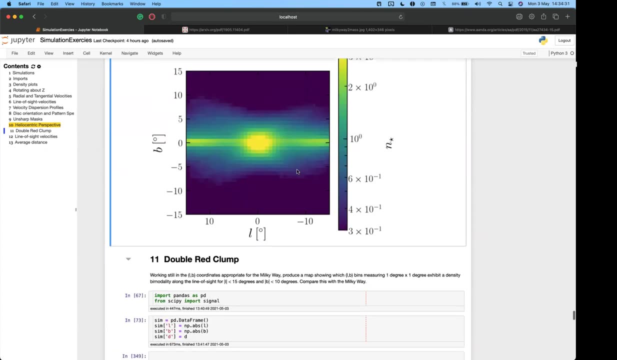 Thank you, I think you managed to mute him. sorry apologies, that wasn't me. The other arm is further away from us because the bar is inclined at an angle, so it appears at lower heights in this kind of angular space. So, moving on to the final couple of things, 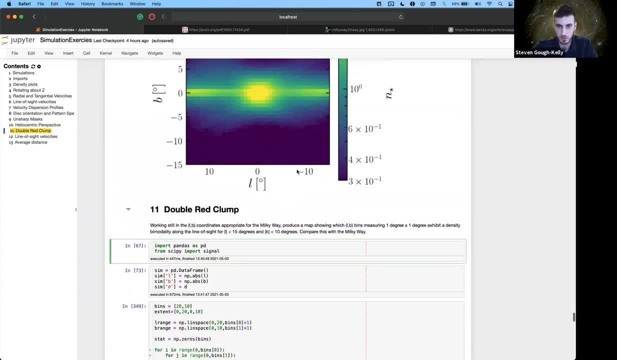 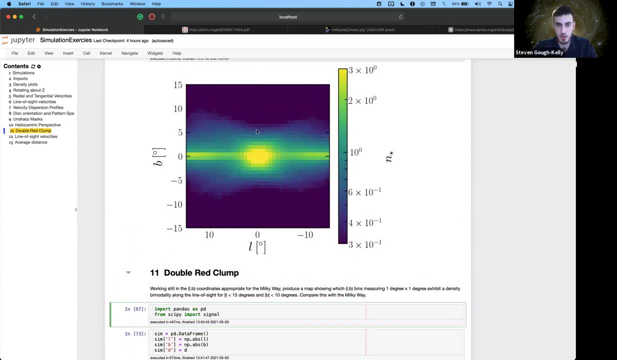 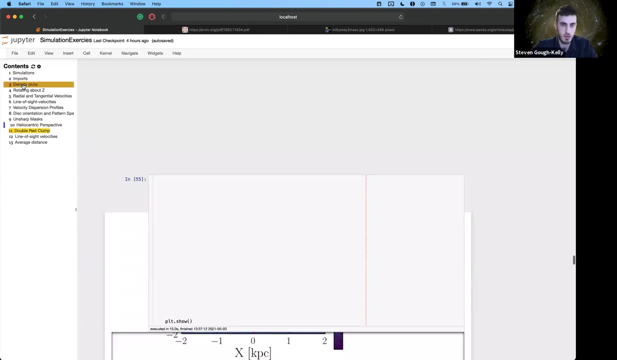 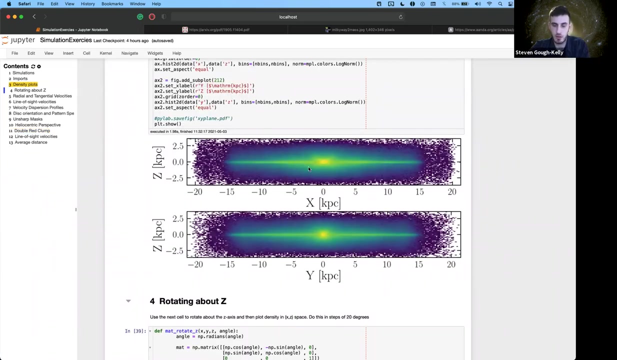 we're going to look at something called the double red clump, which is the kind of a tracer signal of the x-shape within the Milky Way. If you can imagine, let's go to a previous kind of representation. this is the side on orientation of the disk. If you imagine, say hypothetically, 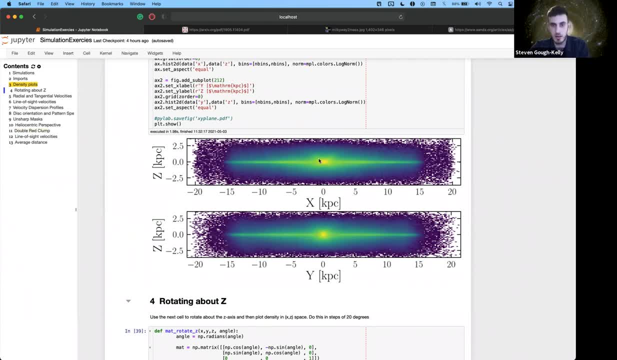 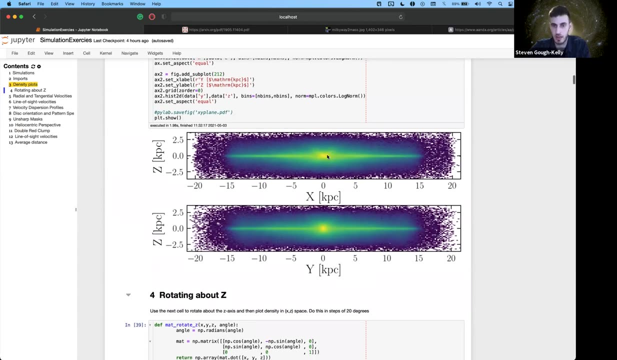 the bar was. we're seeing the bar end on and we're at minus 8x and we draw a line through the x-shape. what you'd expect within the density distribution is an over density here and over density here, corresponding to each arm of the x-shape, Obviously from the bar isn't. 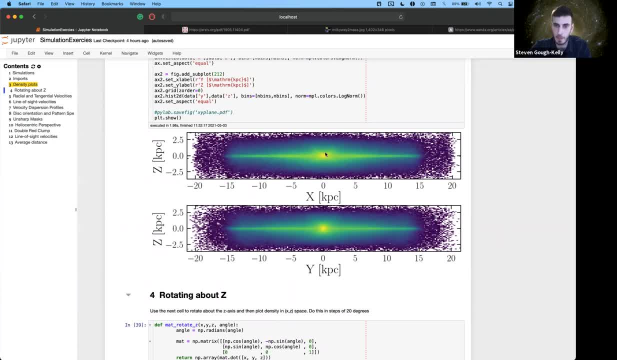 completely end on it's at 27 degrees, so it's a little bit more of an over density, but you don't exactly get one kind of a linear distances. there'll be some level of projection, but you should still expect to find two over. 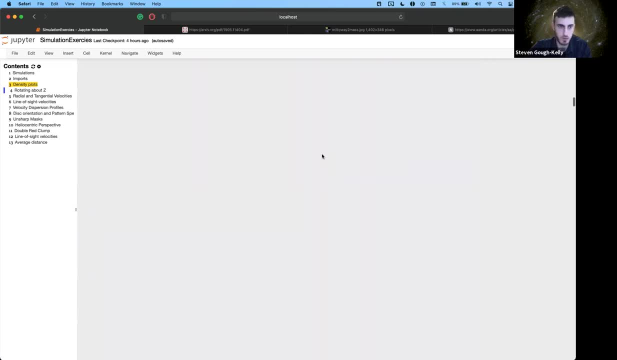 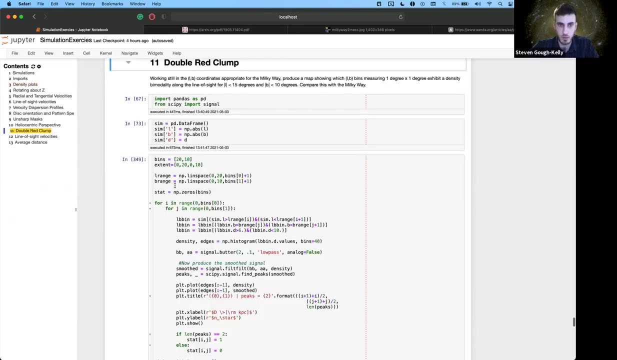 densities along the line of sight. And that's what we've done within the Milky Way and that's what we can do as an exercise in this model. So we're still in LB space and the distance space from the solar perspective. so we're still in LB space and the distance space from the solar perspective. 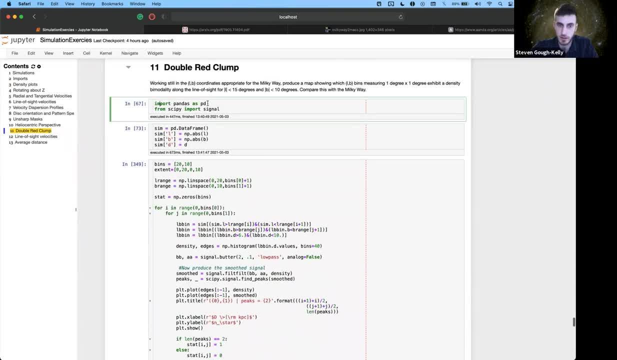 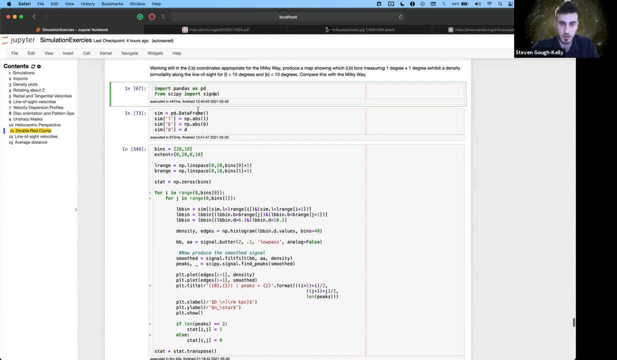 and all I've done here is I'm using pandas just to allow for some storing of the arrays and allow me to kind of index the arrays a little nicely- makes the syntax a little nicer- And I'm using signal from SciPy just to do some smoothing and some peak finding. and I'll show you why. because 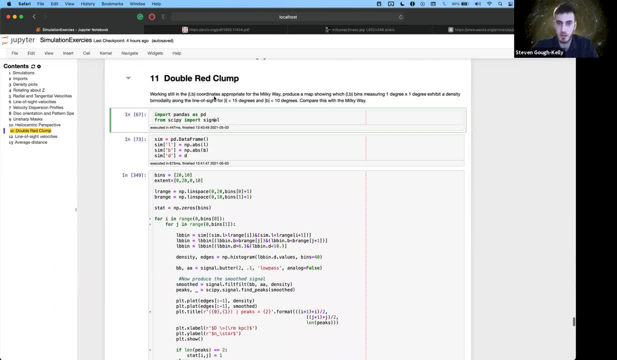 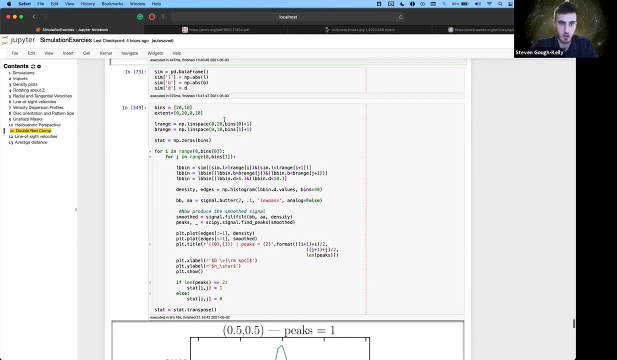 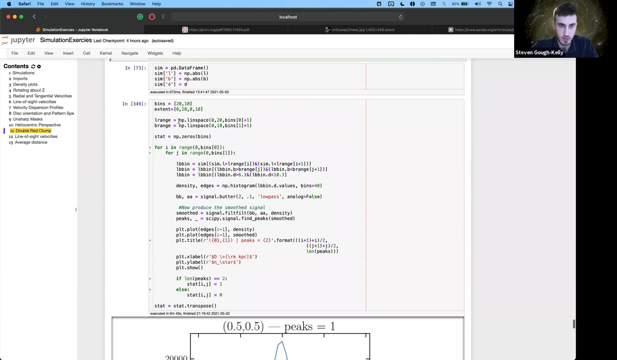 we're going to be looking for one degree fields in the center of the galaxy and we're going to see if we can detect kind of two peaks in the density distribution. So kind of setting that up, I'm just. I'm putting the LBD data into a pandas data frame just so I can index it a little nicer later on. 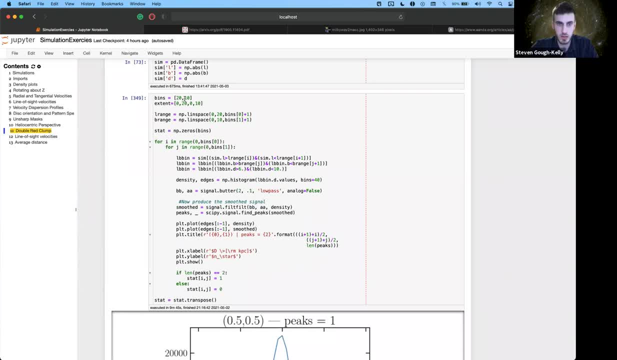 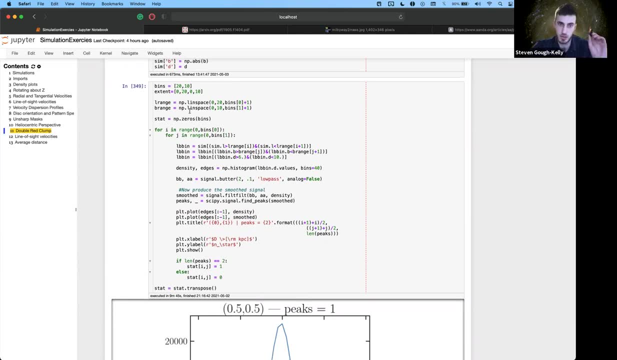 I'm using 20 bins in longitude and 10 bins in latitude, and then I'm going to be looking within that same space. so 0 to 20 degrees longitude and 0 to 10 degrees latitude, and that gives me 1 degree by 1 degree pixels. 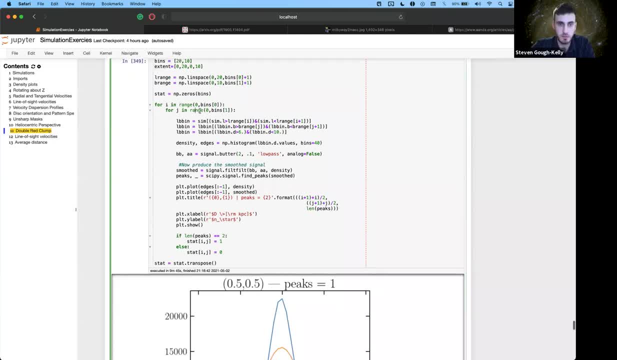 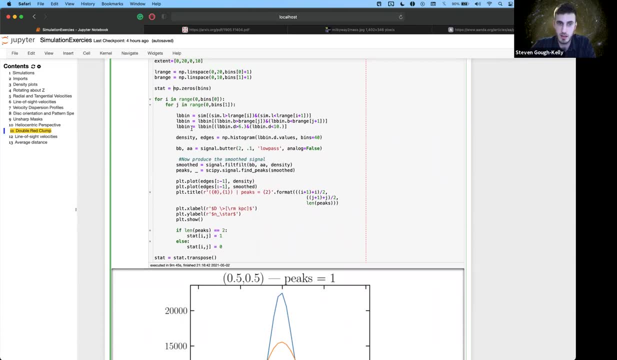 I'm just creating an array to hold some values of the same size of the bins I've just mentioned and I'm going to iterate through each of these bins. It's not the prettiest, it's not the most optimized code you could possibly write for this, but I prefer this method because I can get in the 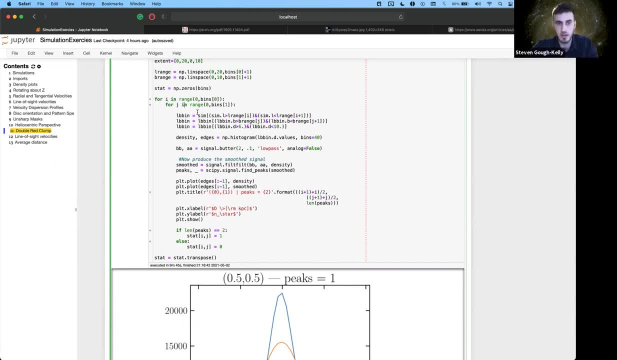 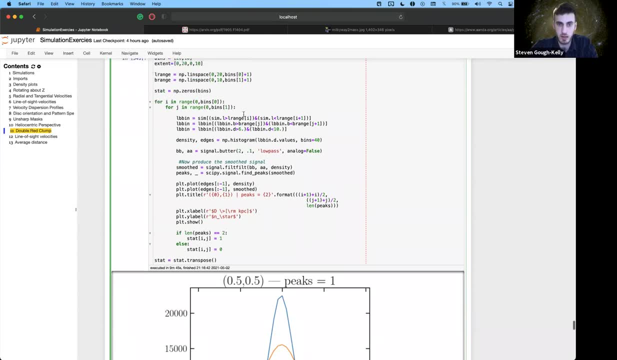 middle of this process and for each 1 degree bin. I know exactly what's going on in that kind of space. So I cut out the full simulation, the L bins and then the L bin that I'm interested in at that current iteration, the B bin- I'm 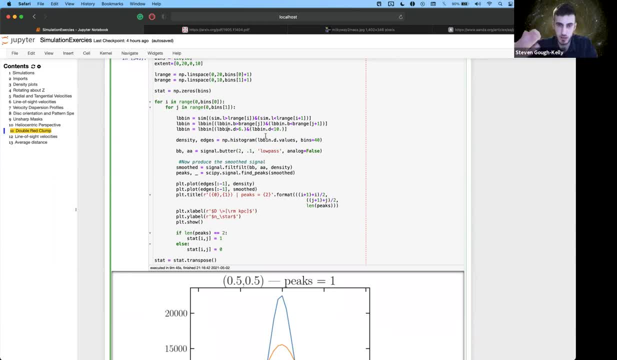 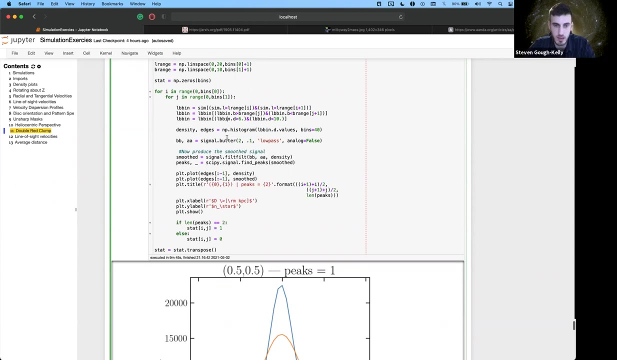 interested in that iteration. I restrict myself to 6 to 10 kiloparsecs, so I'm just looking at the very center of the galaxy. I don't particularly care about the near disk or the far disk, I'm just interested in the very center. I do a histogram of the densities along the line of sight. I then 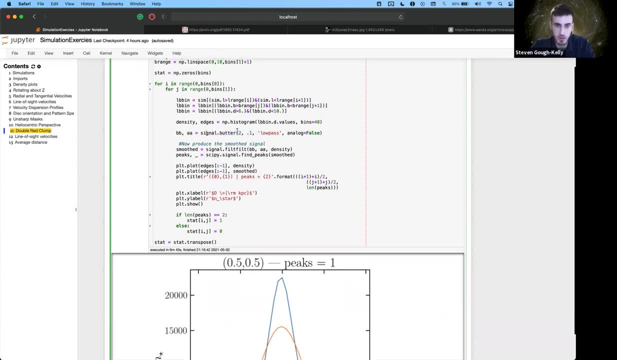 add a smoothing filter to it, because some of them can be a little bit noisy. and then I'm going to look at the density distribution and I don't want to find just low level peaks, I want to find the more general peaks that the X shape would produce. Then I look at the smooths. in fact, get the smooth. 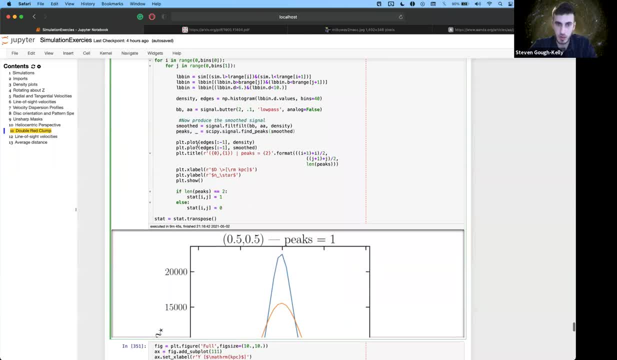 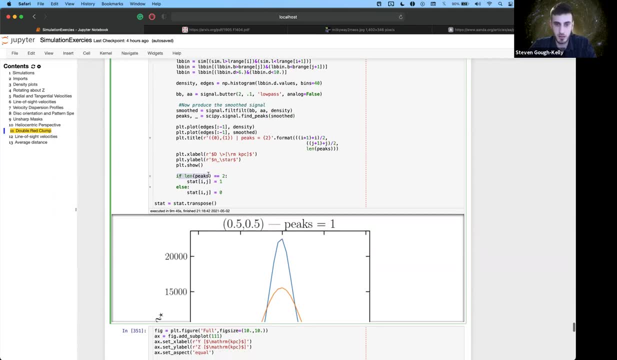 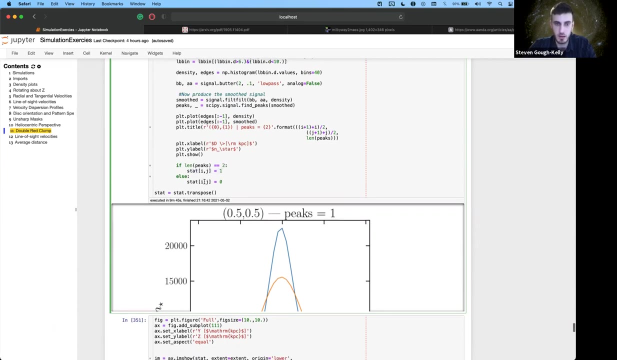 density distribution and find the peaks within it. and then I'm going to just plot out the density and the smooth density just so we can have a look in a moment and show it. And then if the number of peaks in the density distribution is equal to 2, then set the statistic, set the bin, the LB bin. 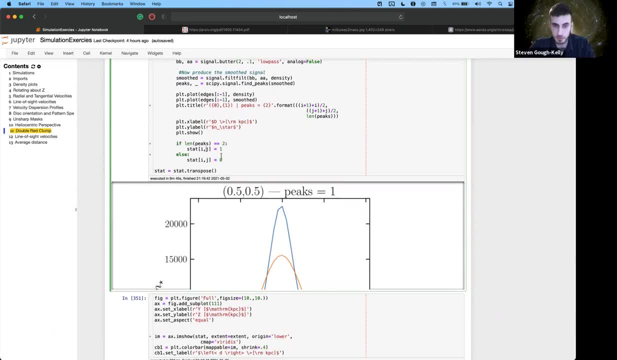 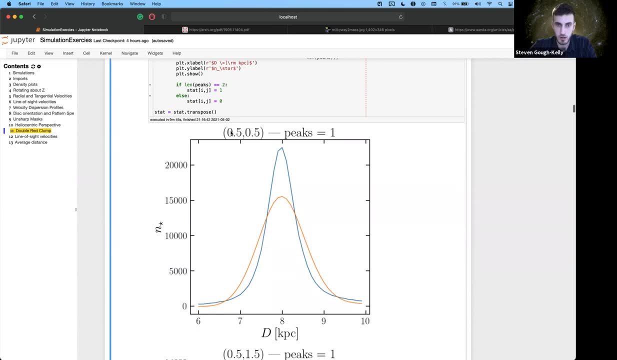 that we're interested in to 1.. If it's not, then it's 0.. So, as we look through a couple of these plots, I'm just going to briefly show you a couple. We've got the longitude and latitude I should. 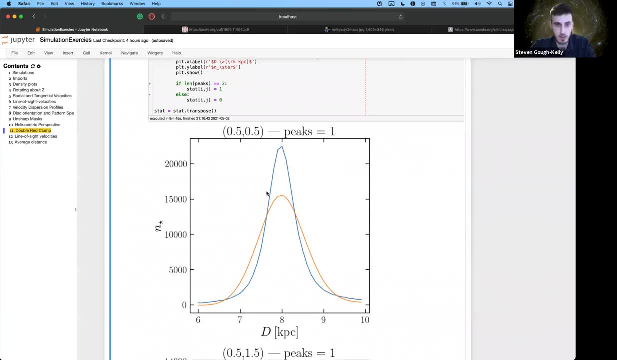 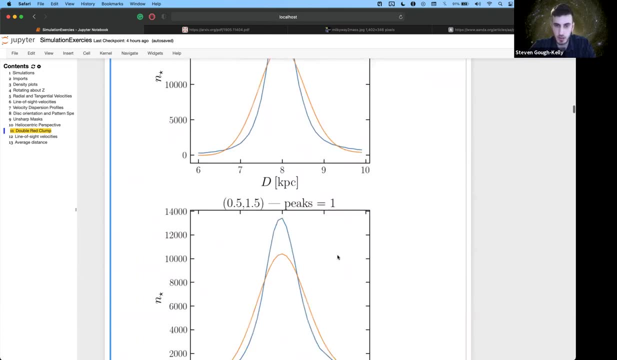 have degree symbols there, but it's me being really- and the number of peaks. So you can see here the blue lines is the raw data and the orange line is the smooth data. As we move through a couple of these you can see that the density distribution gets wider. It's starting to spread. 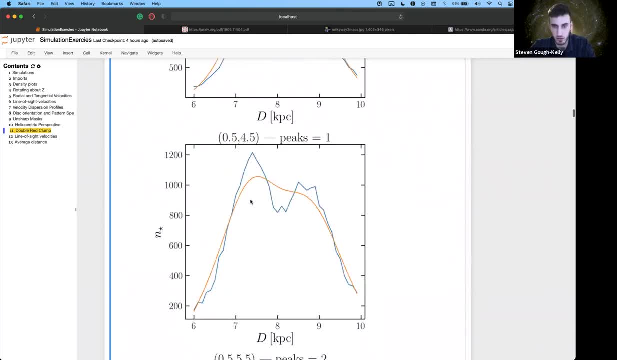 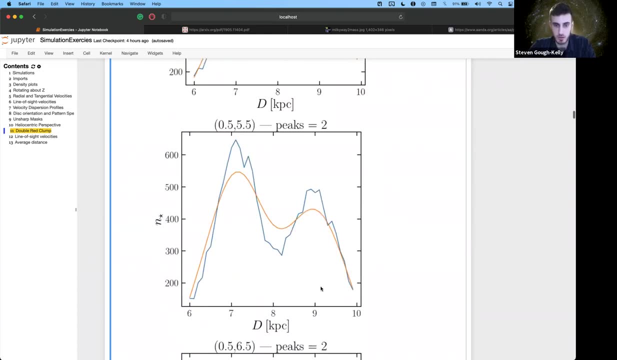 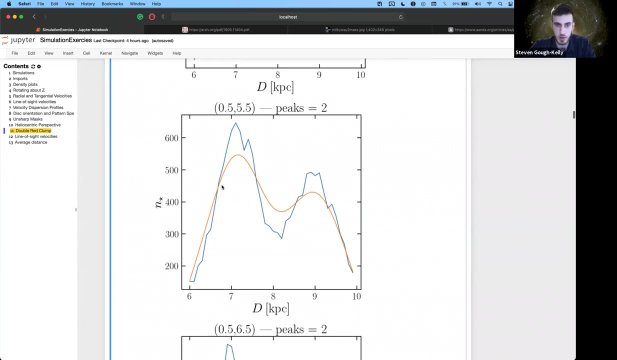 out starting to appear bimodal. I may have over the smooth this a little bit. it's still finding one peak, but eventually you can see the density distribution along the distance. so along from the distance from the sun towards the center, you see that it does become truly bimodal. and there 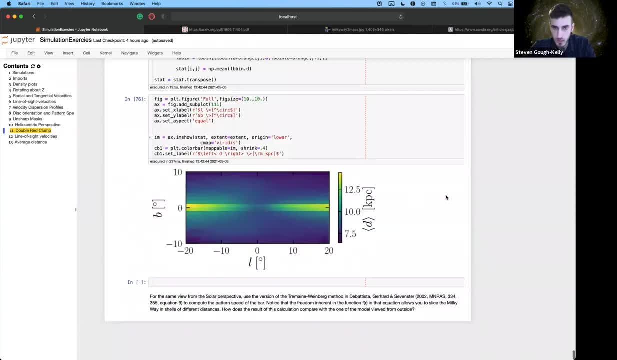 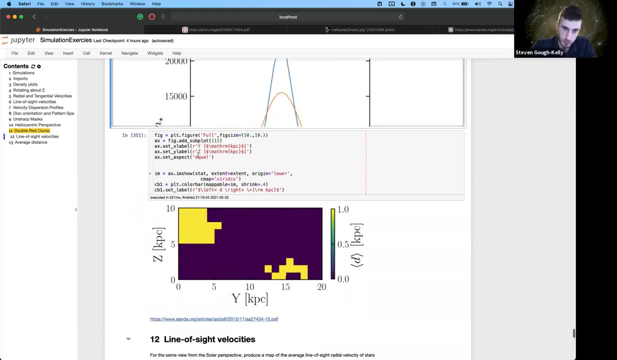 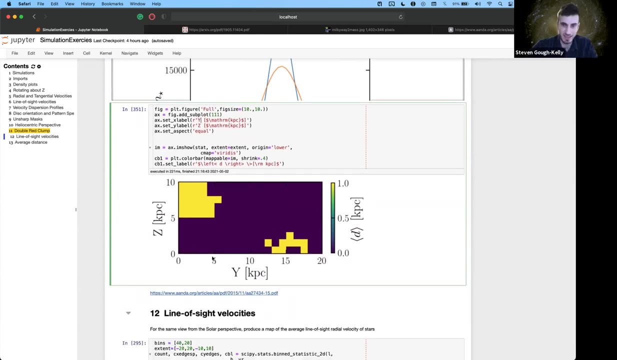 are two peaks and the peak finder detects them. So then, when I plot this as a function of- oh my goodness, this is a function of lb, not yz. see, this is again me being a little lazy and recycling my code. This should be in lb space. You see, the ones that have got the one value in here are on the. 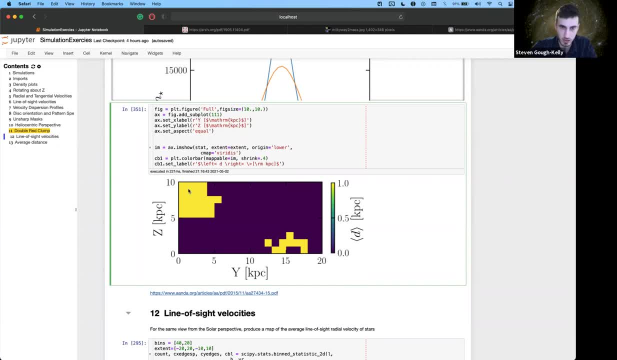 close to l equals 0, so very close to the galactic center and away from the plane, because we don't expect to see the x shape at low down, we expect to see the arms at higher height. And then there's a couple of 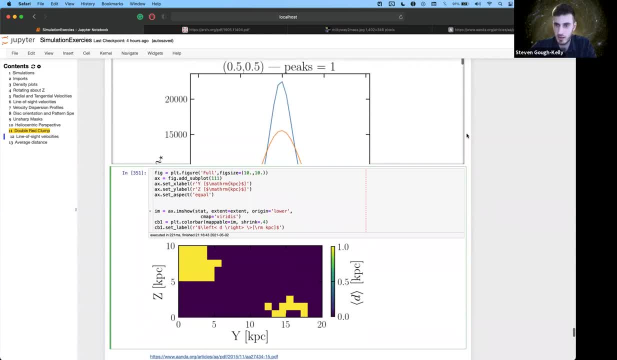 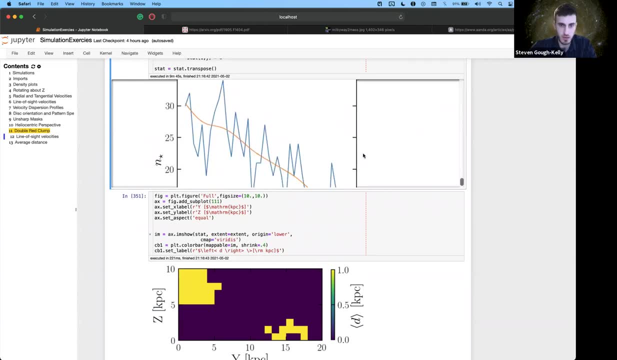 pixels out here which are behaving a little badly, but that's not the x shape. that is just if I scroll down to kind of the bottom here we've got these profiles that have very few stars in along the line of sight, so we're quite away from the galactic center. 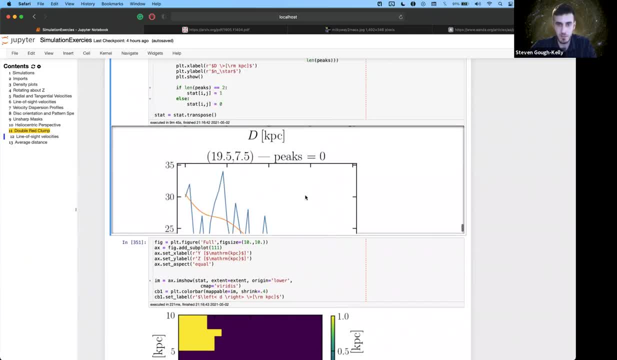 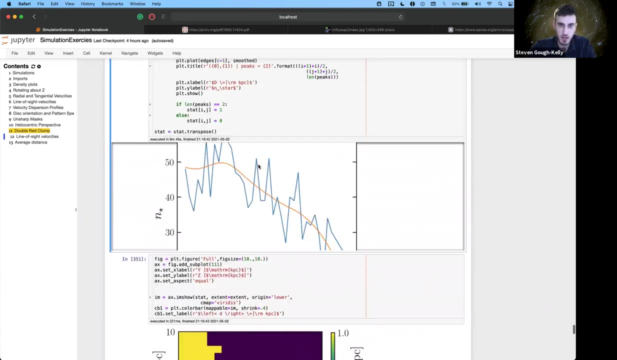 l values over here. So you get some of these values that have peaks, but they're just noise, really, It's not really a true peak in there, and some of these have two peaks. that's triggering this same algorithm. So it's a little bit quick and dirty but it kind of 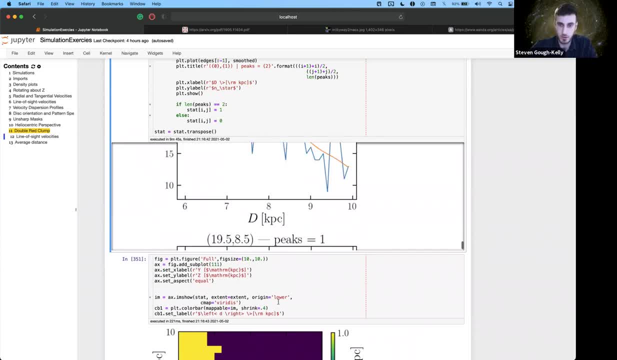 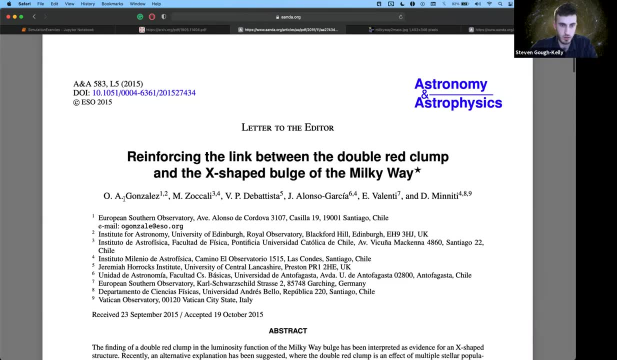 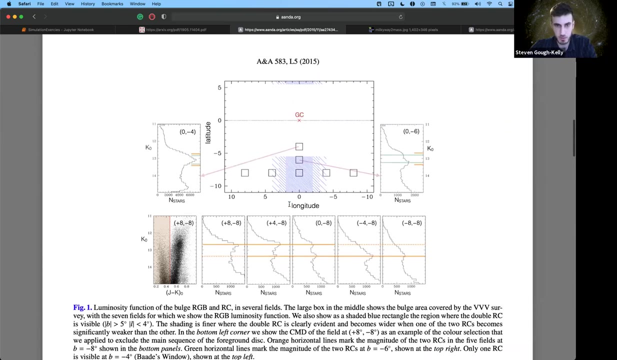 is demonstratory and it shows you kind of what we're looking for within the Milky Way. This has been observed, so you're looking at Gonzales et al 2015.. The reason it's called double red clump is we're looking at a specific type of red giant star that has kind of a fixed magnitude. 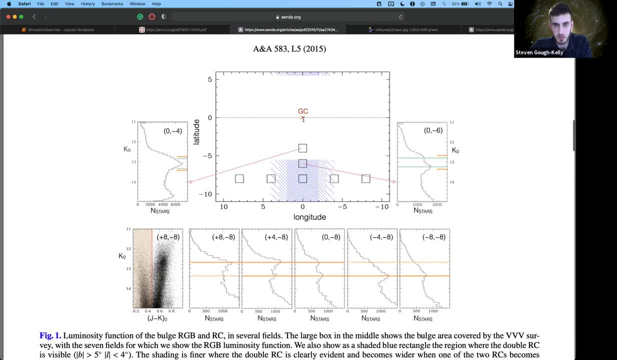 And you can start to see that if we, this is at negative latitude, so this is on low longitude away from the plane. If you go too low, you see the density distribution here has a single peak and as you move out to about minus six you start to get this double peak. 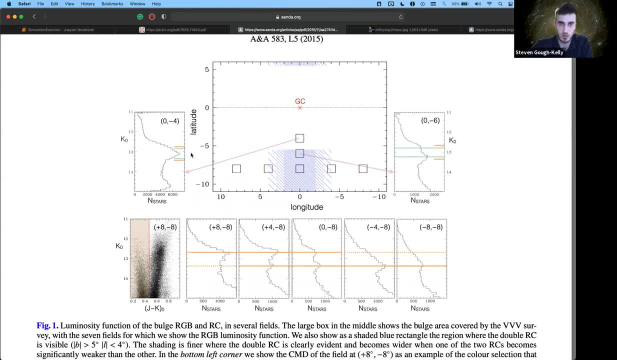 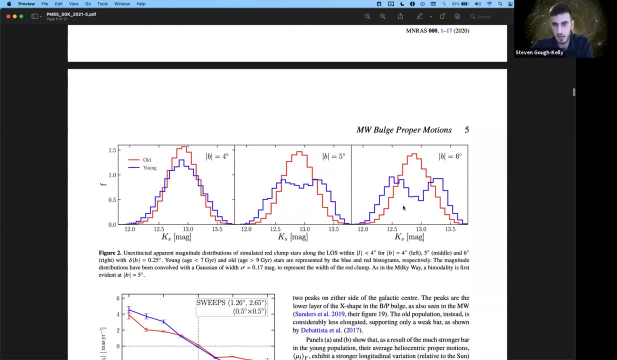 It's exactly what we measure in the Milky Way And it's also- again to plug my own work- something we measure in a different simulation. It's trying to approximate the Milky Way And in the young stars, these blue lines here you can see. 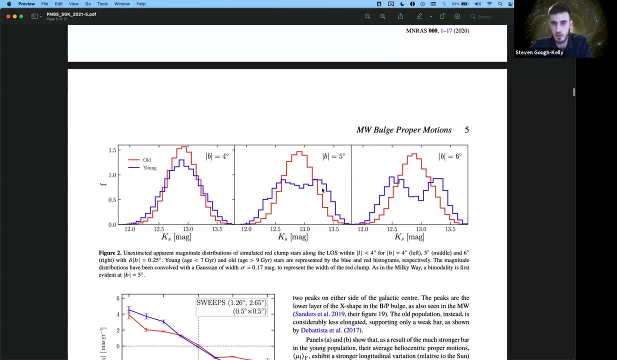 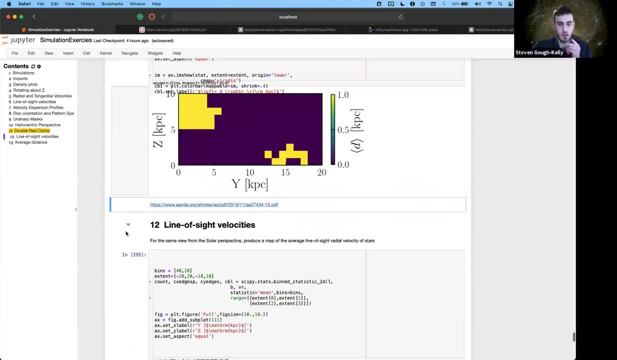 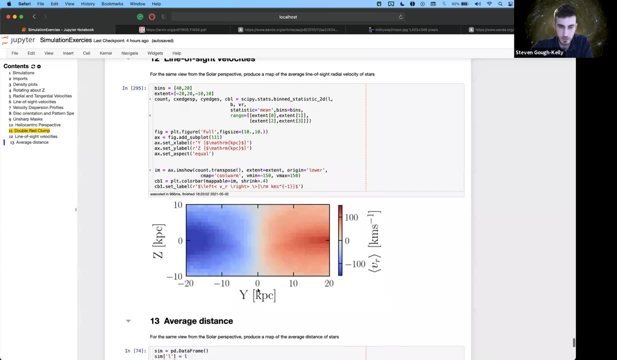 that as you move out to about five and six degrees latitude, you get these double peaks. So let me find my notebook again Cool. So last couple of things: We've got another line of sight: measurement from the solar perspective. Again, my axes labels are wrong. I'm so sorry if. 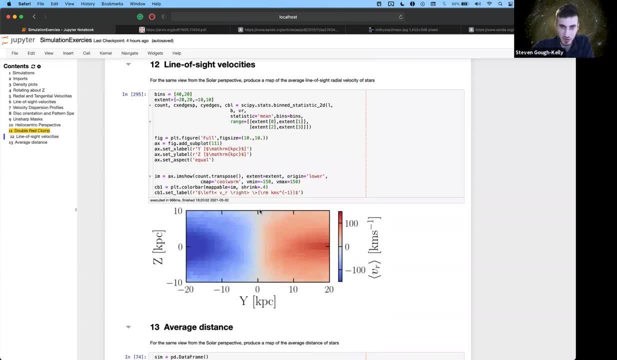 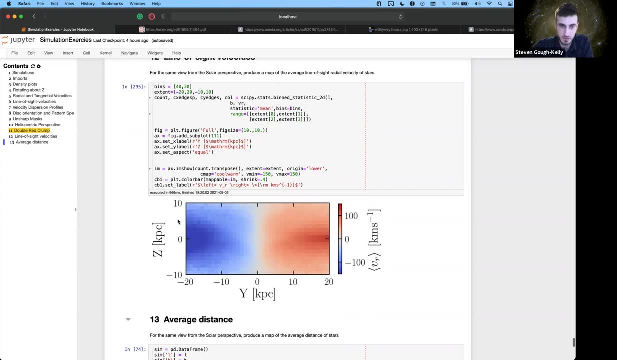 I just try and figure out everything. I'll make sure the rest of the code works And I've neglected the labels sometimes. Well, this is still VR, the average VR. This is L and this is B, And we can also do it for average differences. See, I fixed this one, just not. 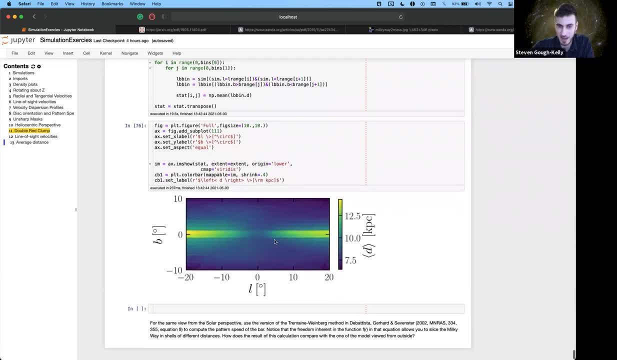 the one above Incredible Average difference distances. So within the plane as you move out away from the minor axis, then you've got- you're looking at more material further away and closer stuff Away from the plane And what you may also see slightly in this plot. 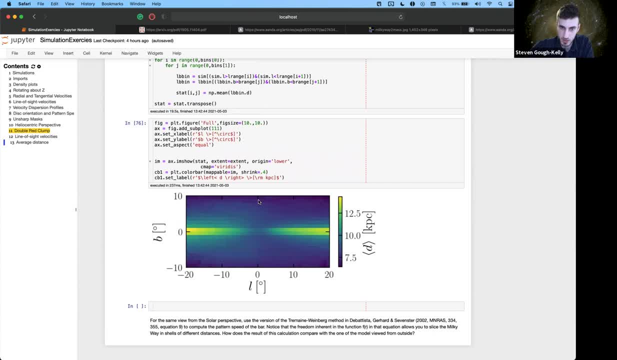 and potentially with the previous plot as well, is because of this kind of projection effect of the bar inclination angle. there is a slight left to right asymmetry in this. It's slightly. Yeah, there'll be left to right asymmetries in this. 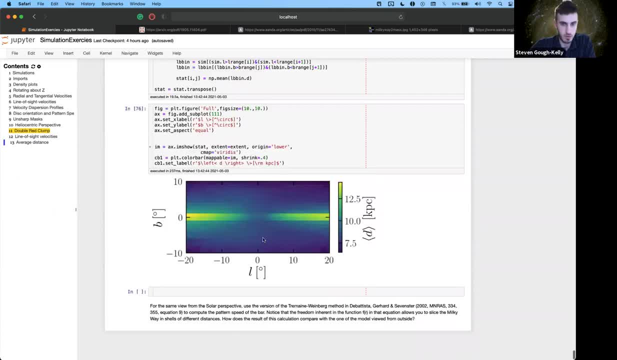 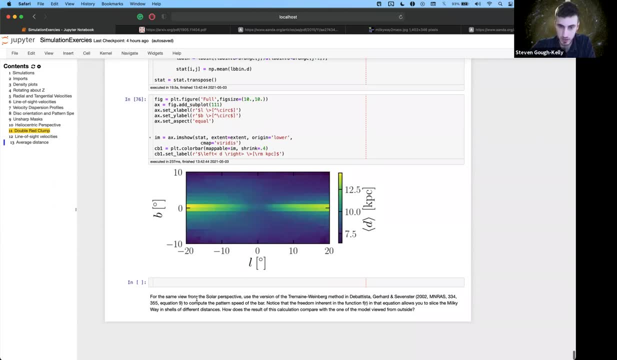 So the final kind of task- I will hold my hand up and say I didn't complete myself because unfortunately I didn't have a chance to fully digest it to be able to write something for you. But effectively it's implementing the Tremaine-Weinberg method from the solar 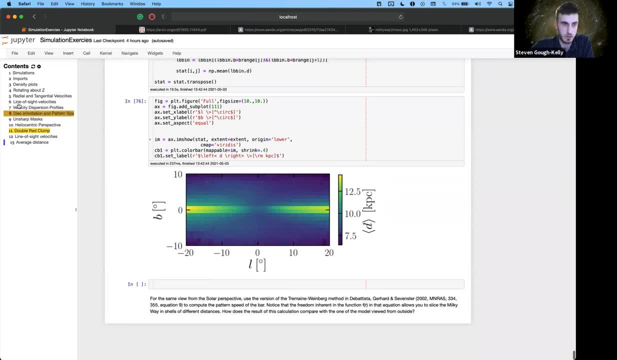 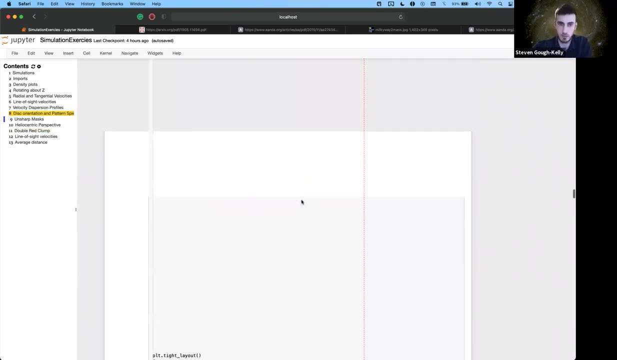 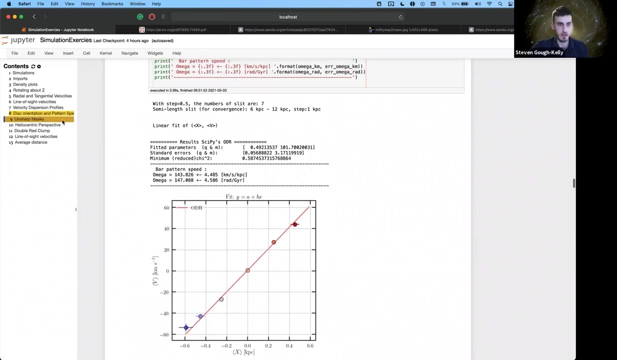 perspective And hopefully if you did this you'd come out with a similar value to the one we measured earlier From the kind of xy position value. So I know I've gone through a fair chunk of that relatively quickly, But hopefully that gave you a taste of how you can start to go through some of these exercises and 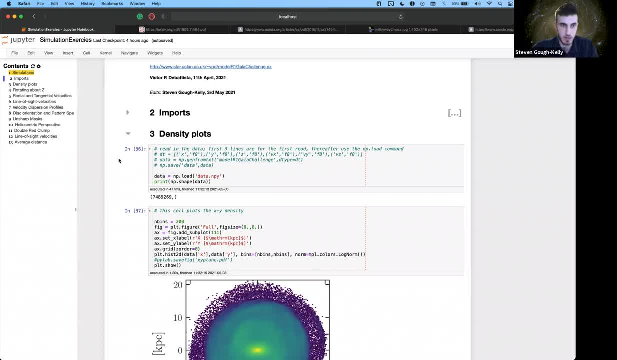 how some of them kind of relate to each other and how some of them kind of relate to the research we're actually currently doing now. But this is just my approach to it. There are many ways to approach the kind of similar problems and many ways to code the same problem. 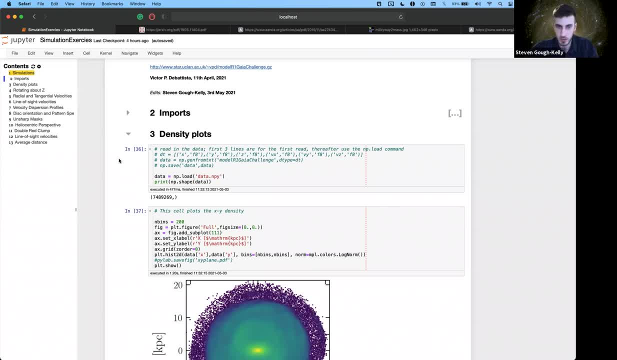 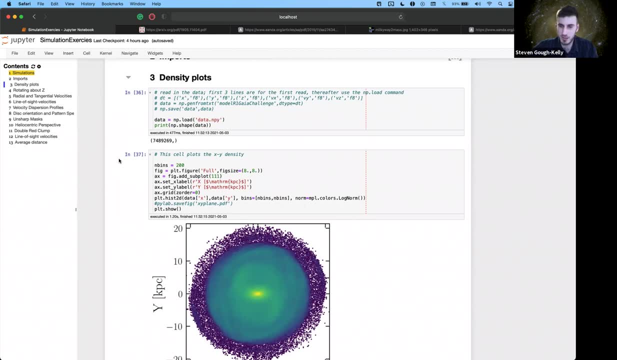 So my approaches aren't gospel in the slightest, especially when it comes to axes labels. Use the correct ones, I would suggest. But besides that, I'm open to kind of any kind of questions of what I presented or if anyone wants to share any of their work. 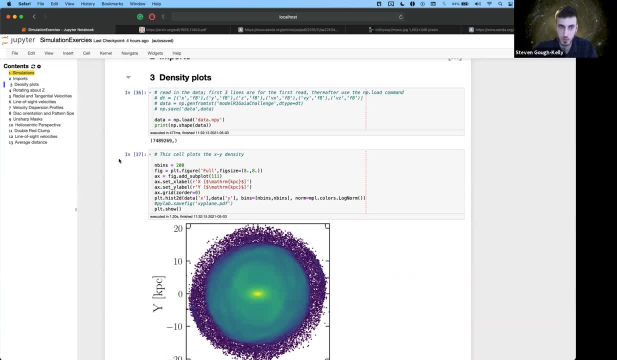 and how they've tackled the same problem or bugs that they've come across, that they couldn't quite come across. But that was all the exercises from my end. So if anyone would like to jump in or if you have any questions, please feel free to share or ask them to me. 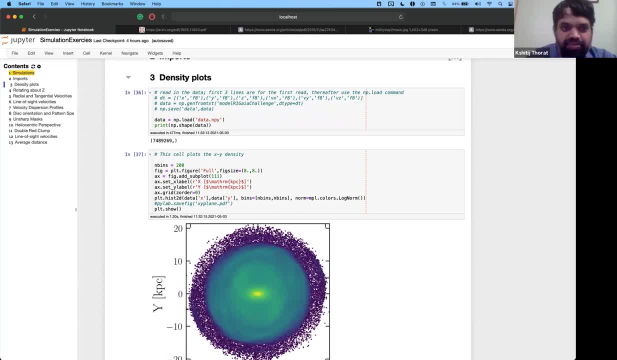 Thank you very much, Stephen, for that excellent presentation and showing us all how to do those exercises. So I agree with Stephen. If anyone would like to share their own way of doing these exercises, or any other questions or comments, please let me know. 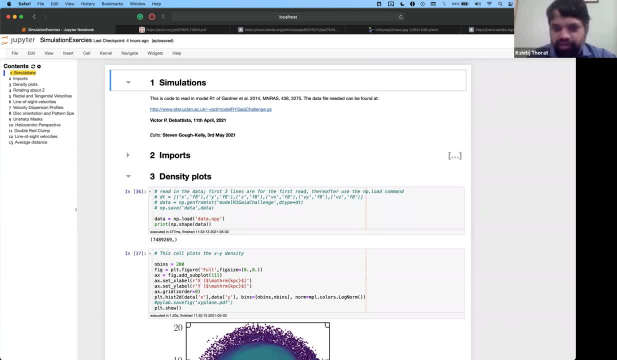 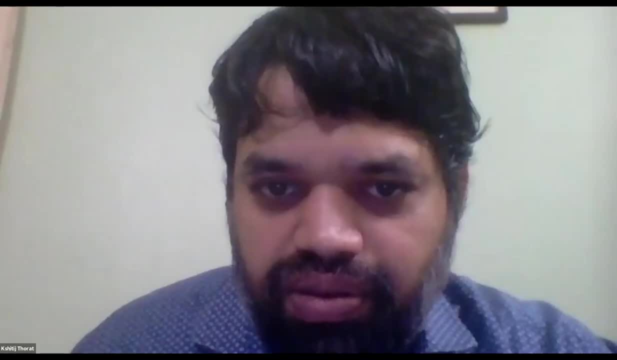 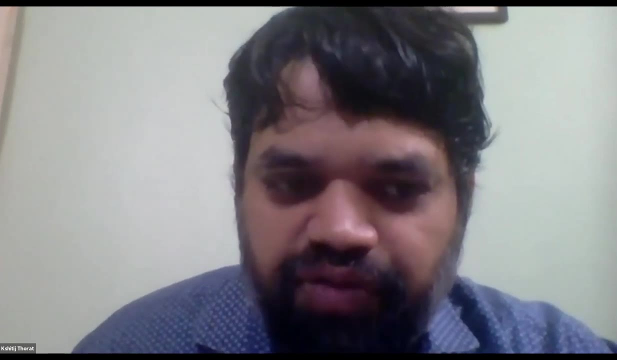 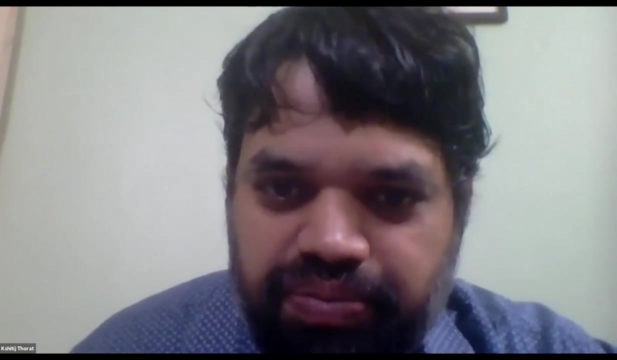 And I can unmute you, or you can unmute yourself and speaker While we wait for the audience. Stephen, could we for a moment go back to the point number 11 in your presentation? Yeah, I was just wondering if we can see the figure. 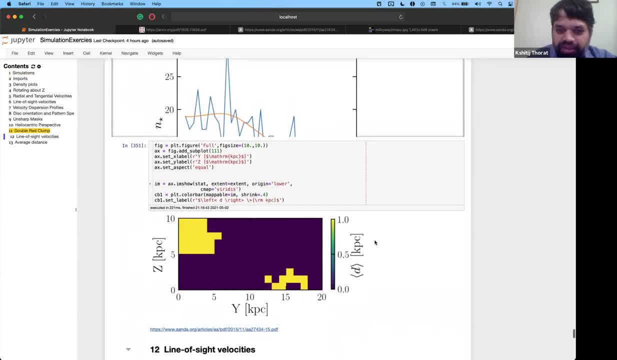 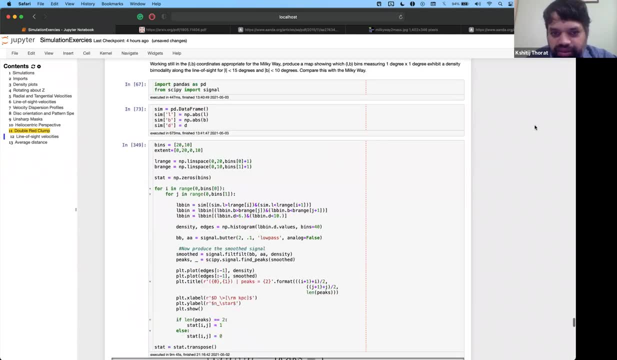 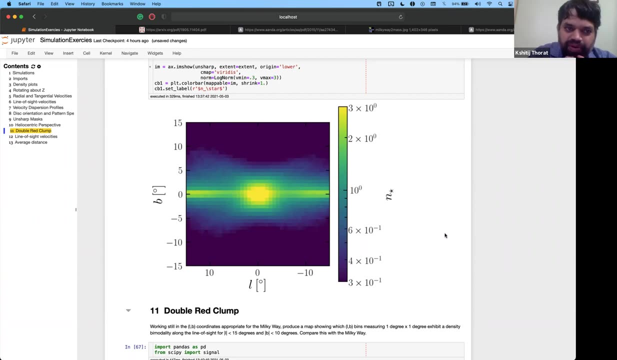 Yeah, Okay, So the figure you were showing. I missed the left. no, not that one. Could you scroll back where we see the left to right contrast? Oh, this sorry. No, I think it was in 11, a bit below. 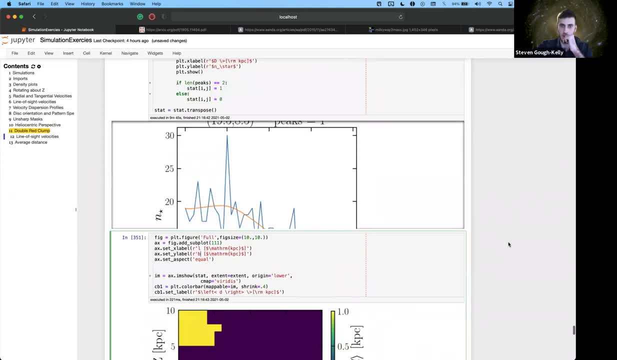 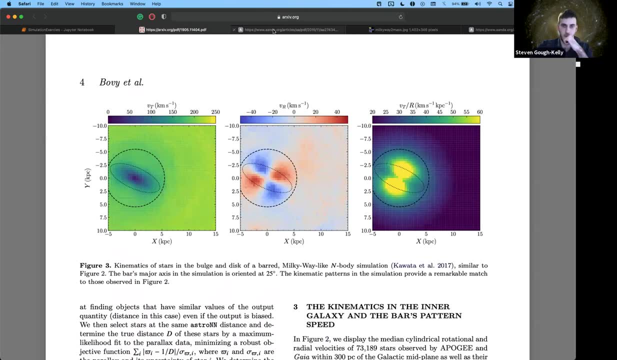 Okay, Yeah, Sorry, I'm not sure which part you want. It's fine, I'll look it up. Oh, you mean from the paper that I was showing? Yeah, Oh, sorry, this one, Yeah, Okay, Thank you very much. 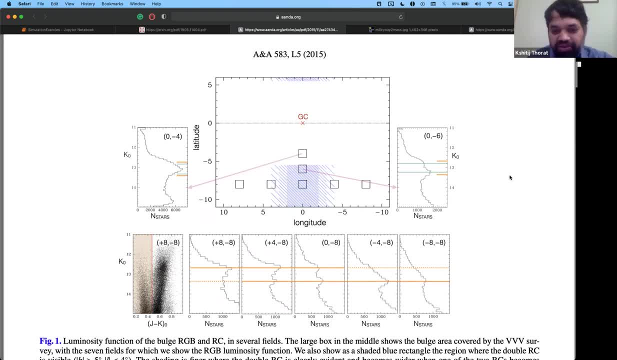 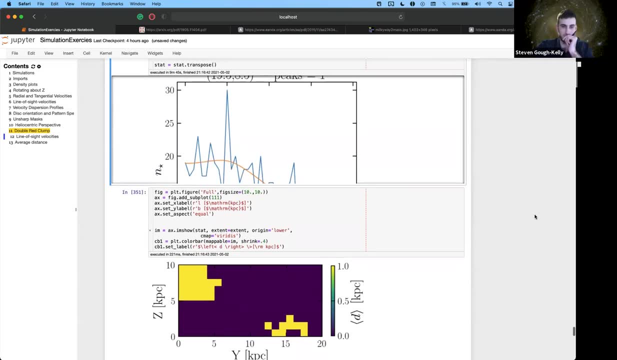 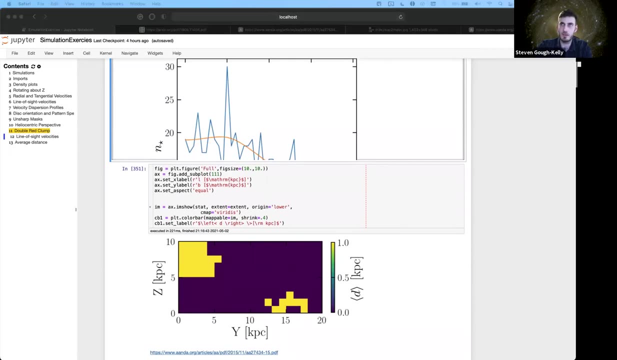 No, I think I have lost the plot which I wanted to retrace. but no worries, Yeah, Okay, Yeah, Sorry, I'm not sure. So would anyone like to show how they have done the this particular exercises? 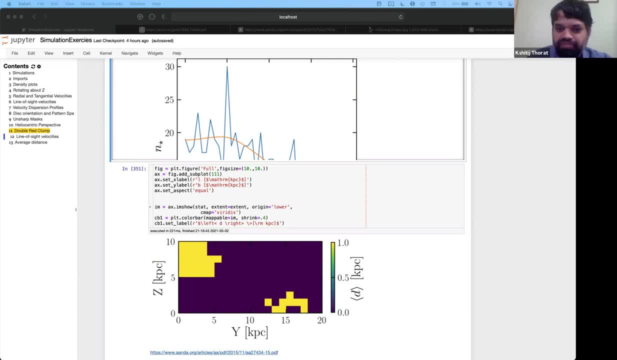 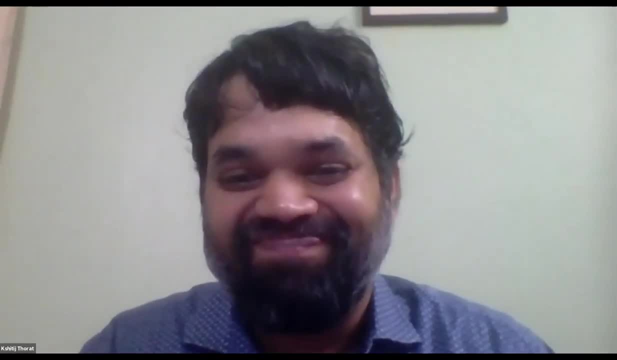 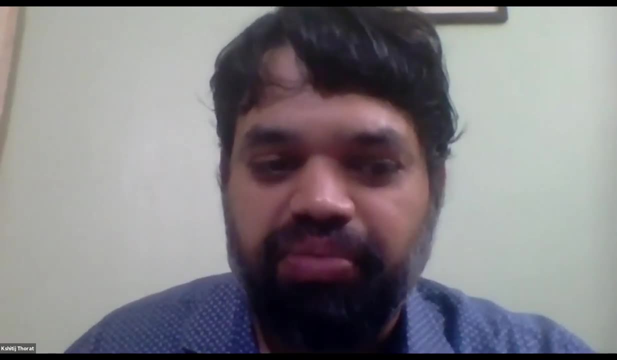 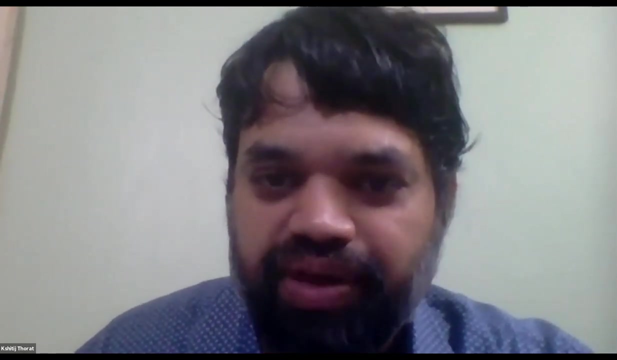